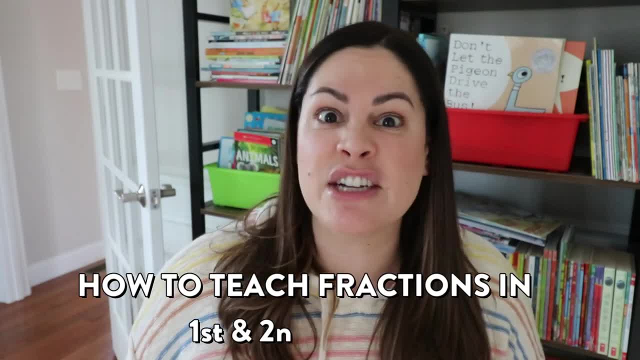 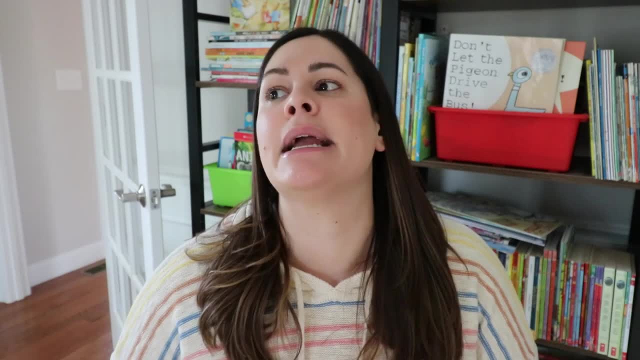 Hey everyone, in today's video we are talking all about how to teach fractions in a first and second grade classroom. Now, fractions tend to be one of those side skills that we teach in the early grades, like measurement and other geometry skills. when we spend so much of our time focusing on 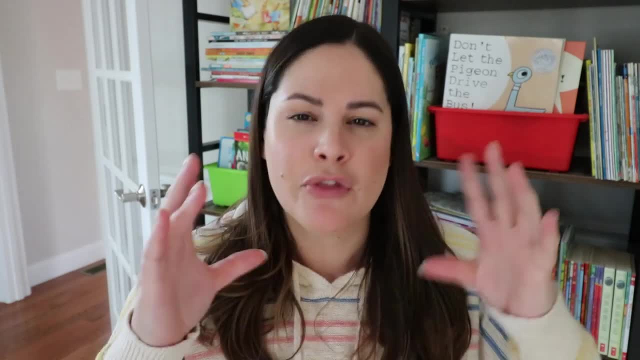 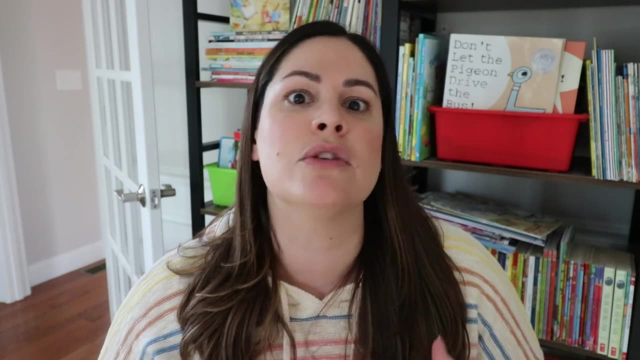 number sense and addition and subtraction and place value. Those are like the main ones. and then we kind of have these side math standards we sprinkle in here and there, but fractions are really one of those concepts that students need to understand as they continue going year to year. 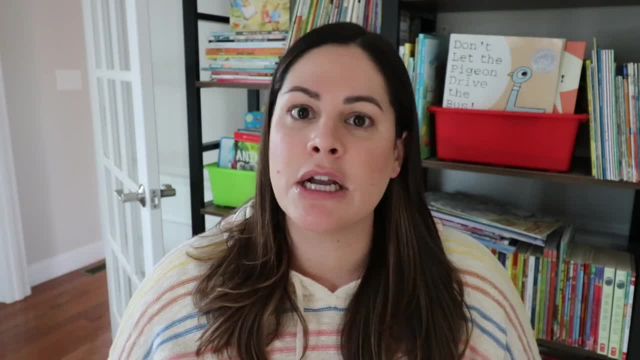 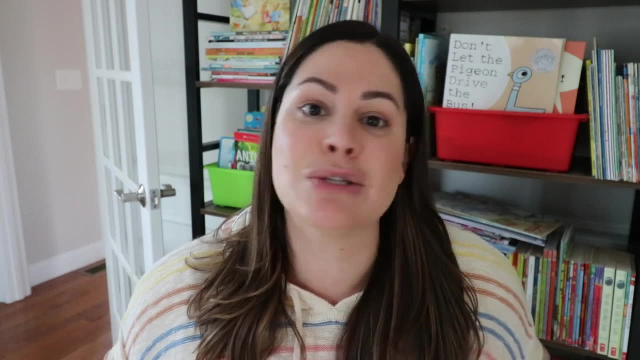 So in today's video, I want to share some of the main things we should be focusing on as we teach fractions to our first and second grade students, and I also have three easy activities that you can use with your kids right away If you're ready to hear what these activities are. 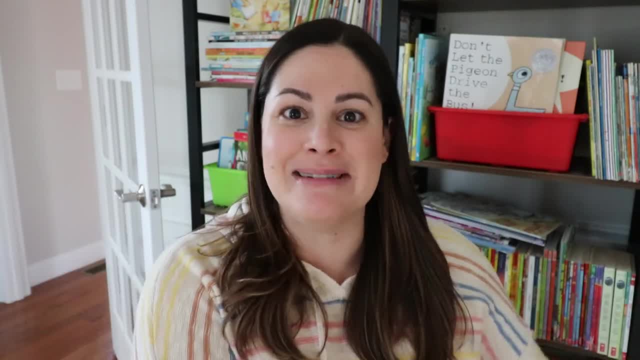 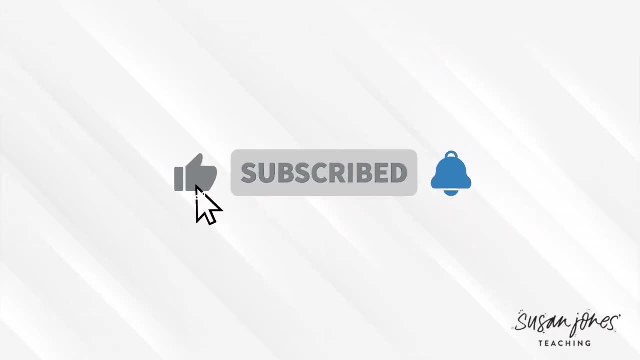 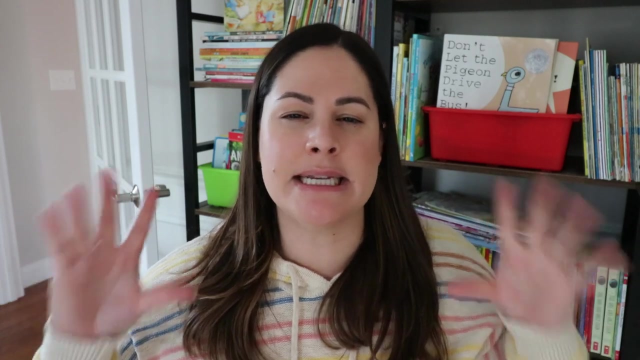 give this video a like, subscribe to my channel and let's get started. All right, when we are thinking about teaching fractions to our first and second grade students, there are a few kind of main points and takeaways that we want our students to understand. 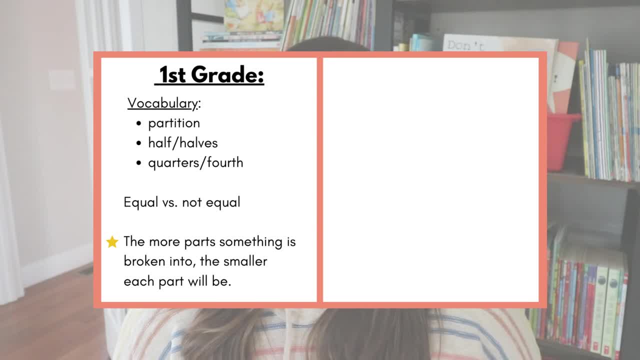 Fractions are introduced in first grade and one of the key terms in the standards is this word, partition, which means, of course, to break into pieces, and I do teach my students what that word partition actually means. So here in first grade, students are introduced to partitioning things in. 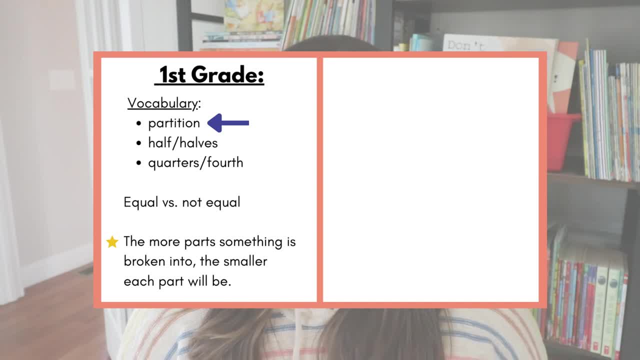 half, as well as partitioning things into fourths or quarters. Now in first grade, we also want students to understand that when we are breaking holes into these fractions of half and fourths, they are in equal pieces. So we do want students to kind of 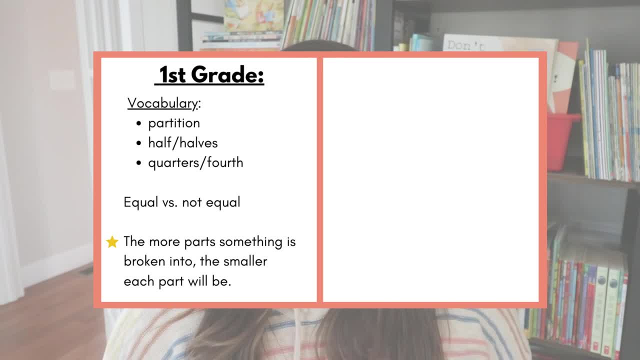 equal versus non-equal. But the big takeaway before students move on to second grade is we want students to understand that the more parts something is broken into, the smaller those shares are going To be. so if we have one half of a cookie, we will have more than one fourth of a cookie. 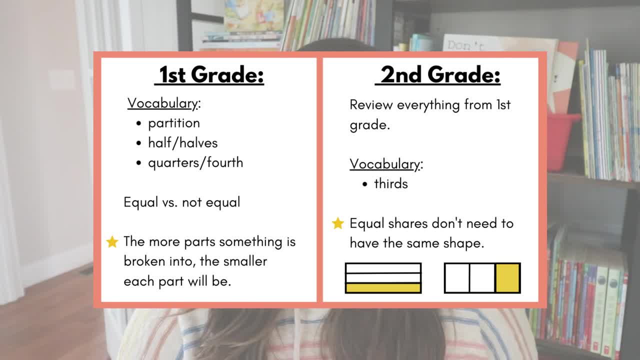 Taking all that information over into second grade, we again want to review partition and what a fraction is. it's a part of a whole, But here, instead of just working on halves and fourths, we are also working on thirds, So they're introduced to breaking something into three pieces. 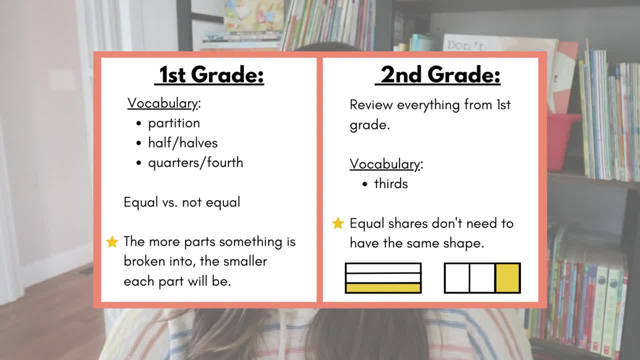 We will, of course, review everything we learned in first grade over in second grade, but the big, big takeaway we want students to leave with is they need to understand that equal shares don't need to have the same shape. Take these two examples right here of 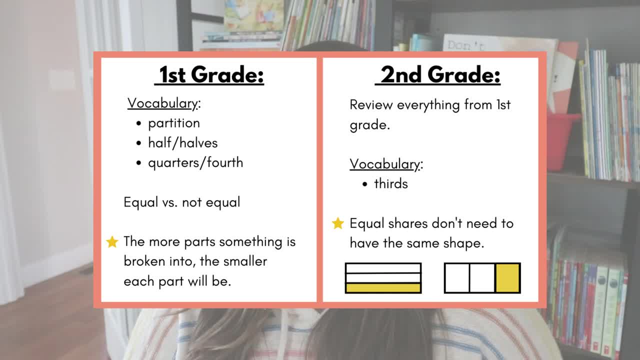 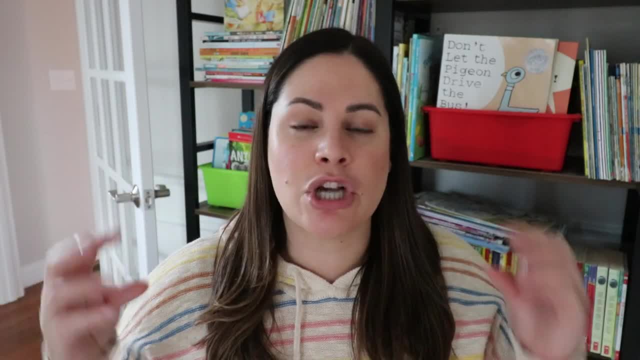 breaking a rectangle into three pieces. They both represent one third, but they don't need to be the same shape. So if we keep those main ideas and goals top of mind when we are teaching fractions to our first and second grade students, there's something kind of glaringly missing that I want. 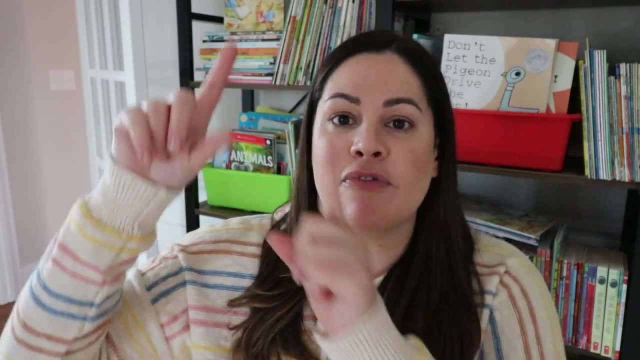 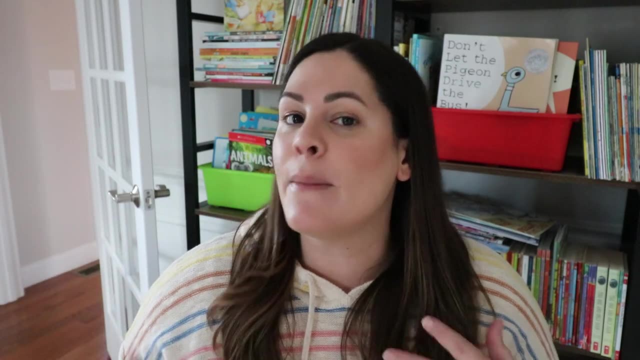 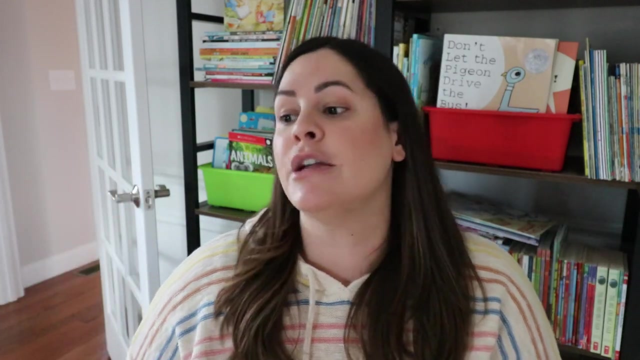 to point out, And that is that the actual numeric form, the abstract form of a fraction with a numerator and a denominator is not shown. right, That is not mentioned in the standards. Now that doesn't necessarily mean that you don't want to show students what that is, that you don't want to. 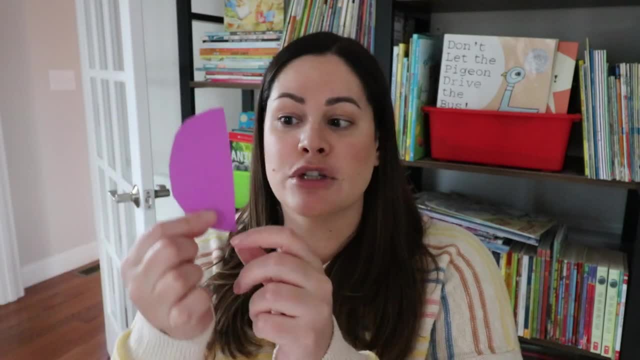 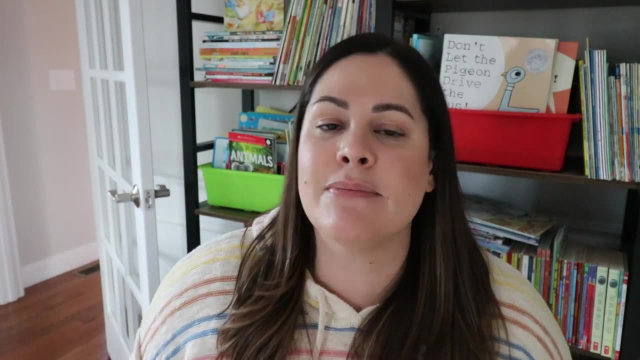 show them half of a circle and you know once we've learned it for a bit and then we can show them what one half looks like when written down. That's totally fine to do, but it means students don't need to master that and you don't want to muddy the waters per se early on when teaching fractions. 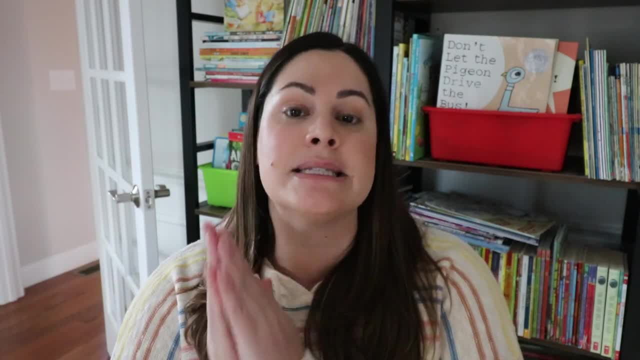 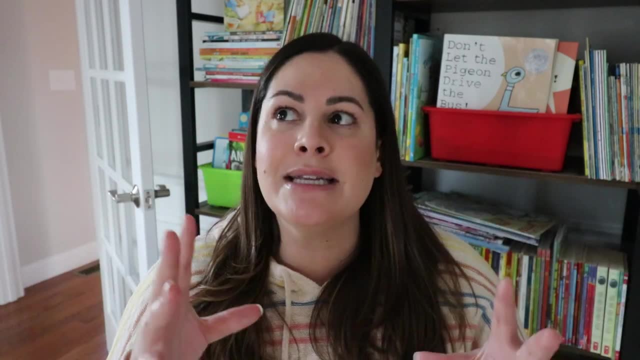 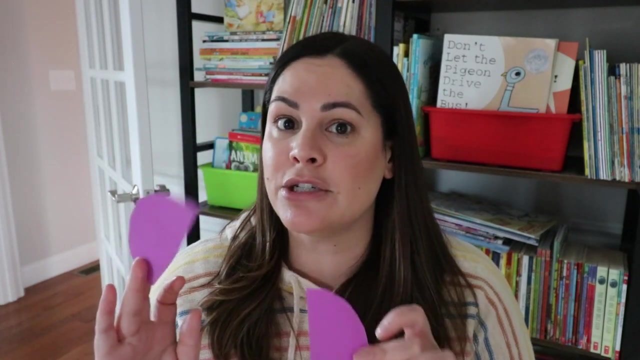 What this also means is we know, with math we want to teach using the CRA model, working from concrete to representational and then to abstract. So what this means is, when we think about the standards in first and second grade, we are largely sticking with the concrete and the representational. And just a side note, 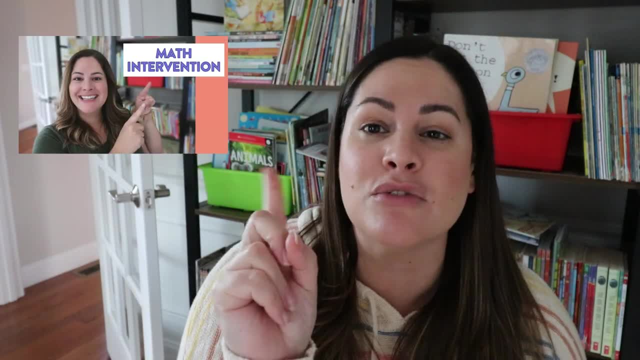 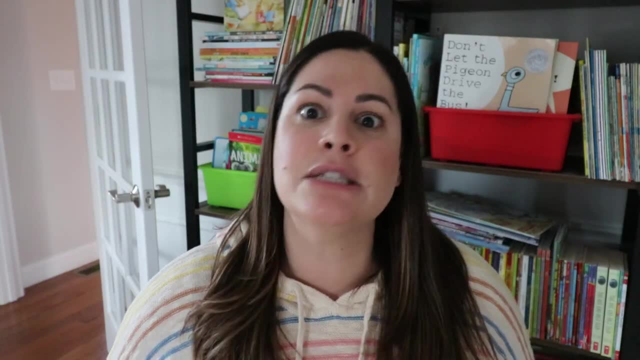 if you don't know what I'm talking about with the CRA model, I have a whole video on it right here. It's one of the best research-based math strategies for teaching your students new math skills. What this also means is we don't need students to look at a whiteboard and compare. 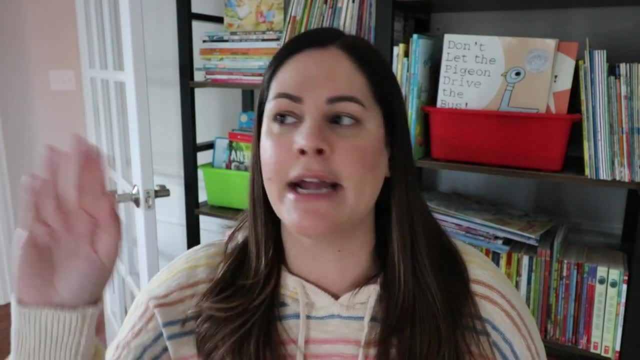 their math skills. We want to teach using the CRA model, working from concrete to representational and then to abstract. So what this means is, when we think about the standards in first and second grade, we are largely sticking with the number one to one half, without any visuals. Right One, one half. 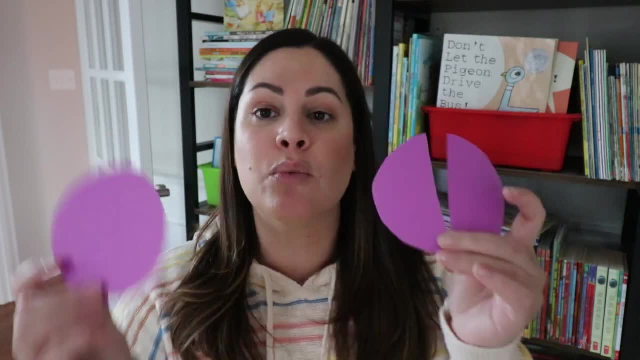 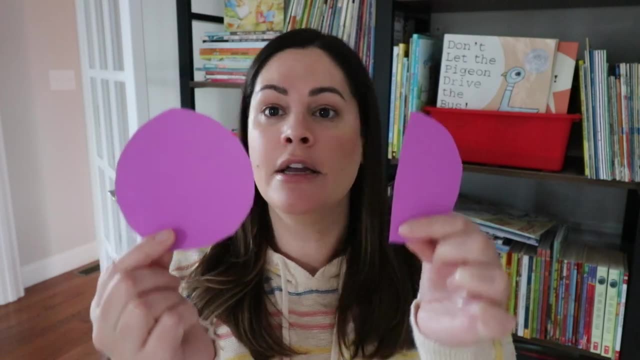 which is bigger. Students do not need to do that, However. I would like them to take a look and see this piece and this piece and recognize which is bigger. We can say: this is a whole, this is a half. which one is bigger. and how do you know? Now, 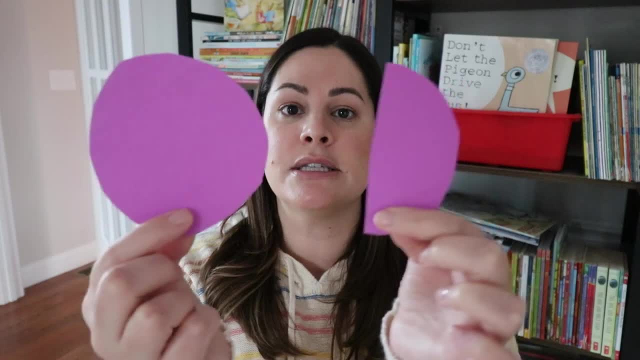 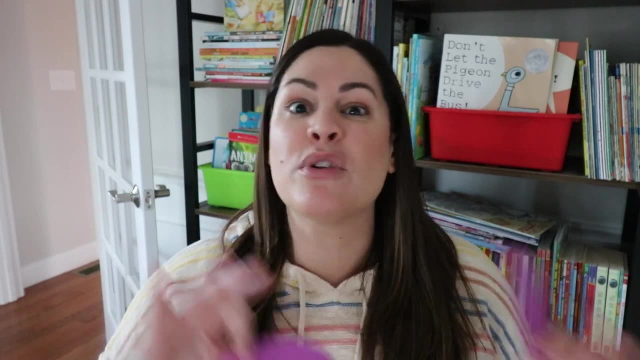 so here they are comparing it. but remember, this is representational, This is concrete, They can hold it And this is where we need to lay that foundation and get students to really understand concepts before they move on to trickier fraction concepts later on. All right, so now that we 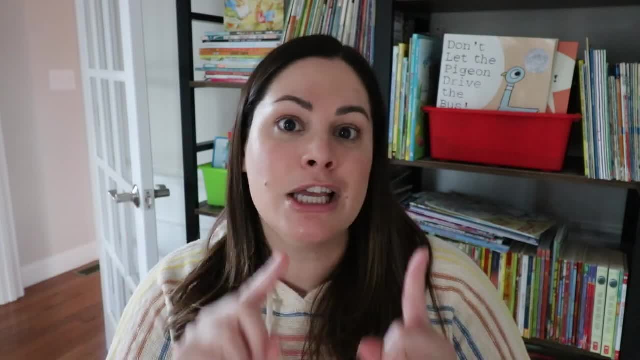 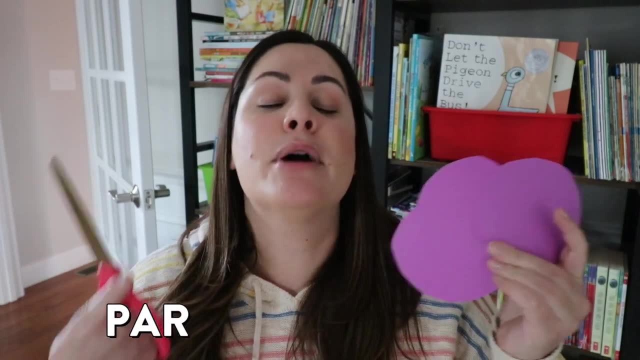 understand all that. here are three different fraction activities you can do with your students. The first one is as simple as some scissors and some paper. Here we want our students to actually partition objects. Now, when I am introducing fractions to my students, I like to do it with 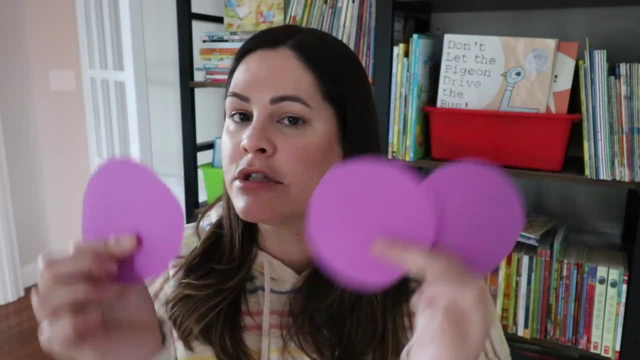 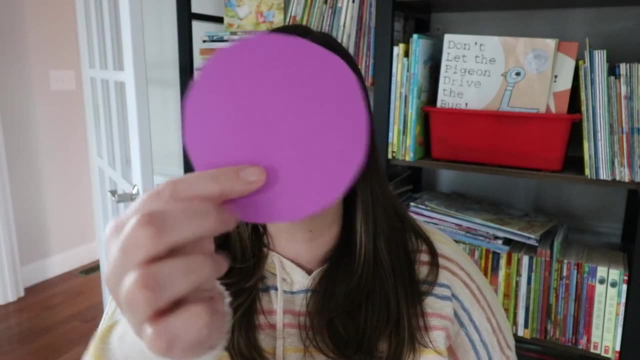 three big circles. Now I will go ahead and have three circles on construction paper, but I will also make sure that all of my students have the same three circles. Now I kind of eyeballed this and my circle is not perfect. Just FYI, I would go ahead and probably print out some circles for 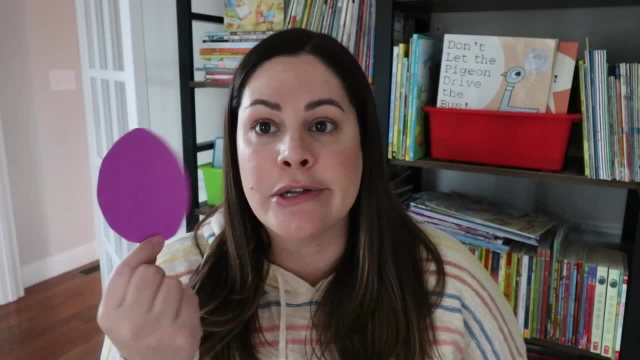 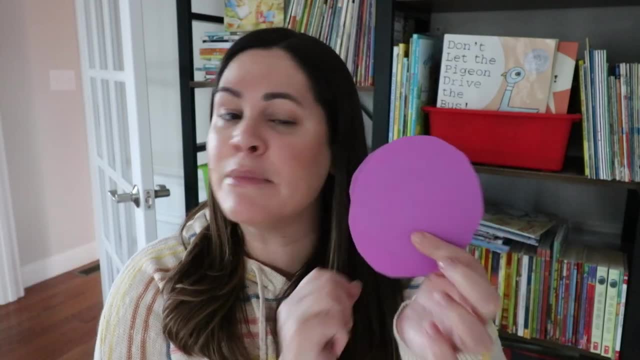 them to cut out on dotted lines, because I could barely do it myself and so having kids, you know, eyeball cutting out three identical circles would be a little difficult. So step one is just some simple, fine motor practice: Have them cut out three identical circles. So once you have your circles, 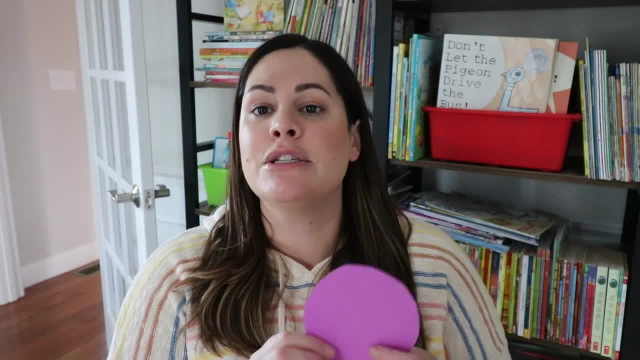 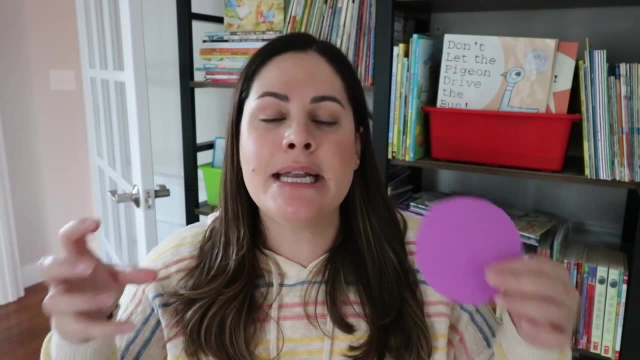 in front of you. this is where I introduce the lesson. I tell my students: here we have one circle, right? I want to go ahead and split this circle. I want to break it into pieces so that we have two equal parts. How can I do that? This is essentially going. 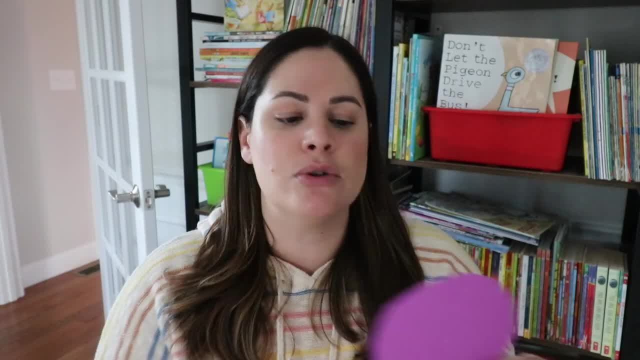 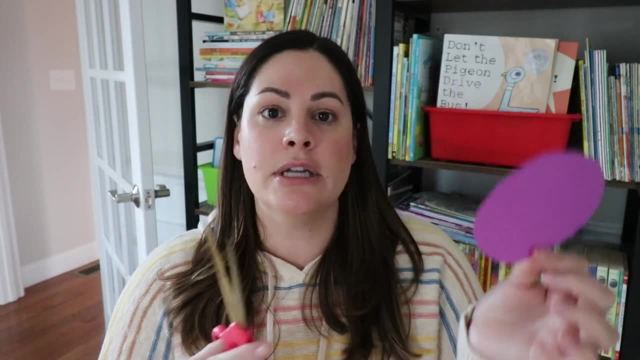 to be a guided math talk, where I am listening to the students and guiding them towards the answer before we do it. So I don't just give students the scissors and the circle and tell them: okay, go ahead and cut this into two equal parts. We talk about it first and then they watch me do it. 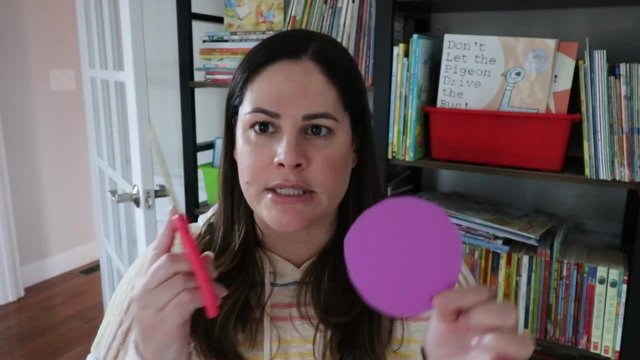 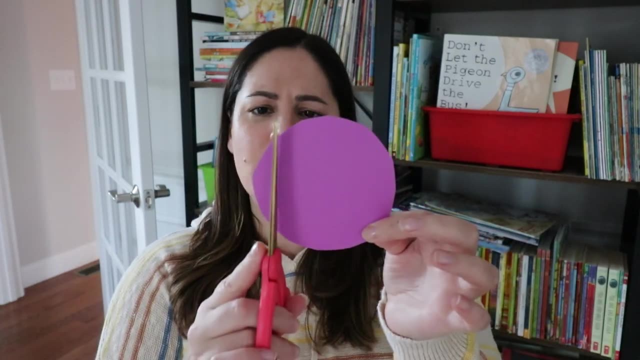 before they do it themselves. Sometime throughout this you know talking it out process, before I've actually cut the circle and I'm still gathering ideas, I will say: okay, so we want to cut the circle. you're telling me What if I go ahead and cut it right here And I show them a non-equal 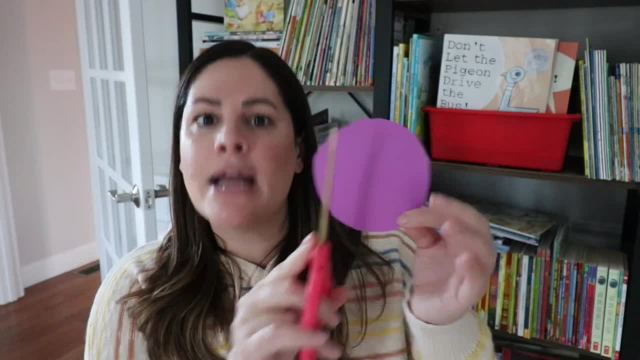 example, right, And they'll say no, no, no, you can't do that And I have them explain why. Oh, if I put the line here or if I cut it here, this side is going to be smaller than this side. Okay. 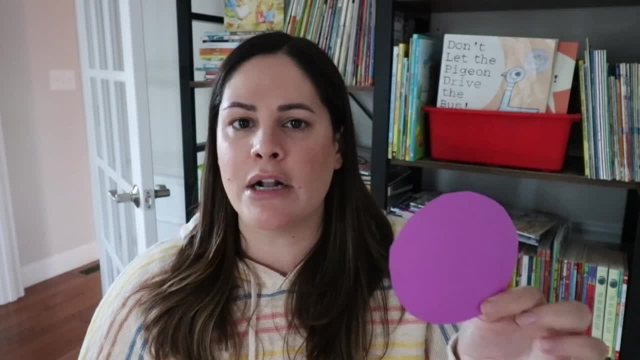 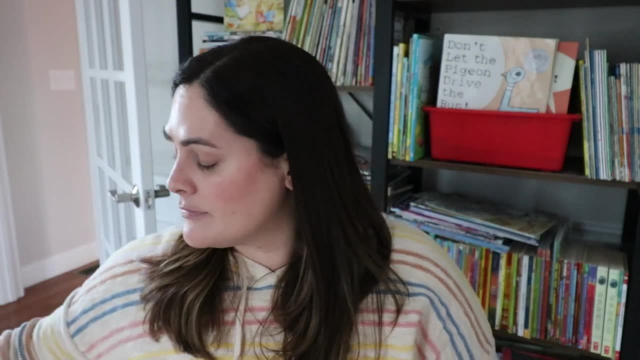 okay, so where should I do it? And we'll determine where it is in the middle. Then I will go ahead in front of the class or under a doc cam and I will cut it into two equal pieces. Not that one went flying, but I have another one right here So and I can show them again. I didn't, I eyeballed. 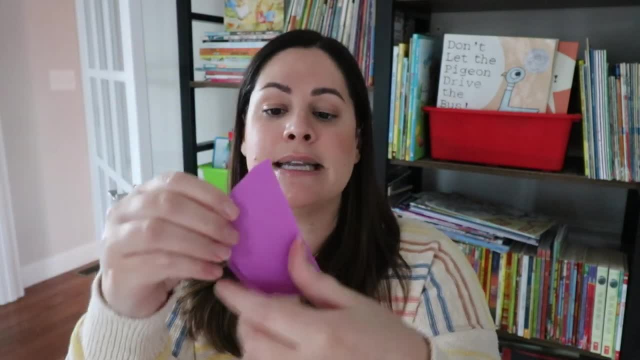 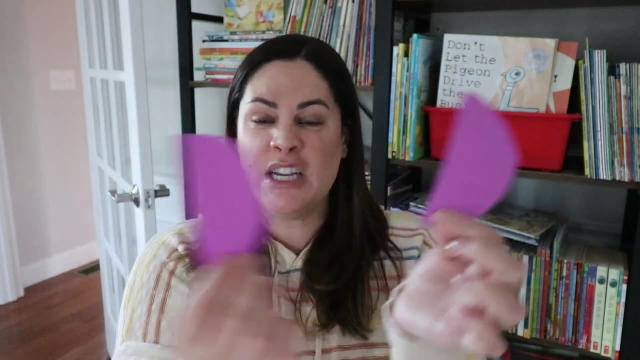 it. but if we actually went ahead and drew that line, they should be nice and equal. And then I would ask my class: you know, would we be happy? Let's say we were going to split it and you got this half, Would you be happy? Yeah, it's equal, I'd say so. And after you cut yours, your students. 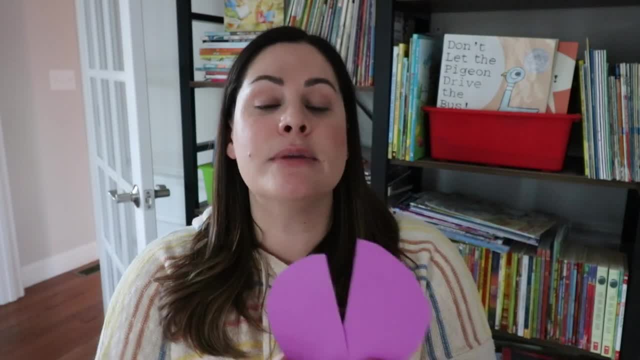 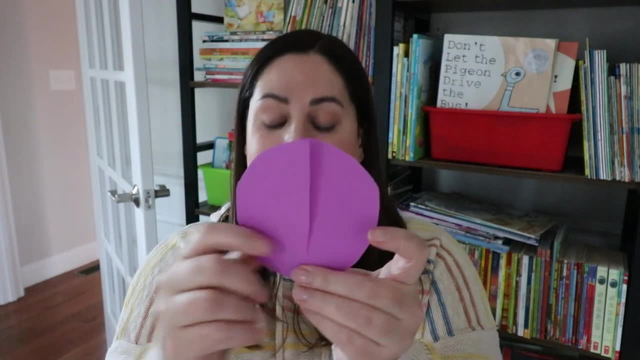 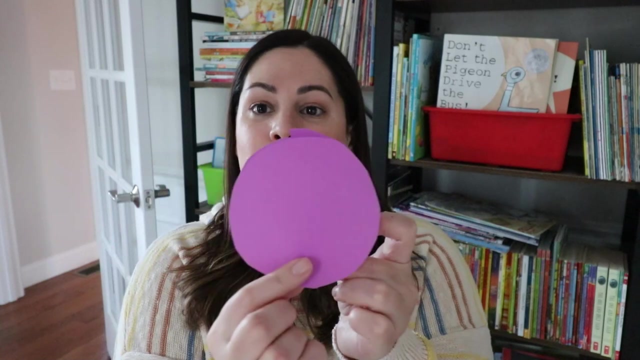 will follow suit and they will do the same thing. This is where I tell my students. we cut that circle in half And when we look at each of these parts here, these parts represent the same amount as this. If I put these two halves together, I get a whole. It was the same because they have. 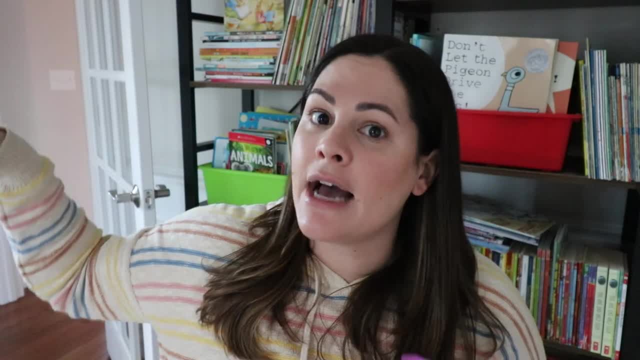 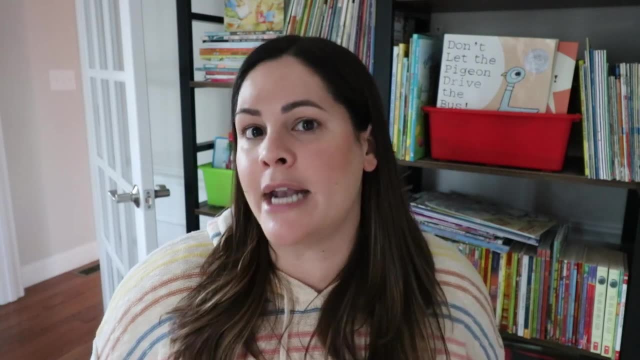 their other circle to compare it to, And during this time I will write the word half on the board and explain: this is one half of a circle. I will then ask my students to hold up one half of a circle, and they will go ahead and hold up one half. I will ask them. 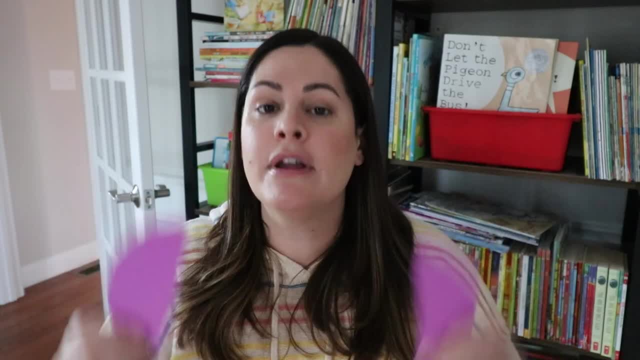 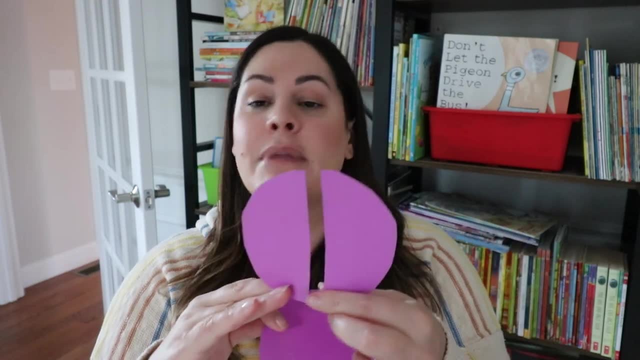 use half in a sentence. I cut my circle in half. Here is one half of a circle In this type of talk it through lesson. not only did my students learn some vocabulary, maybe you told them to partition the circle in half. They used half. They got to see what a half looks like. They talked 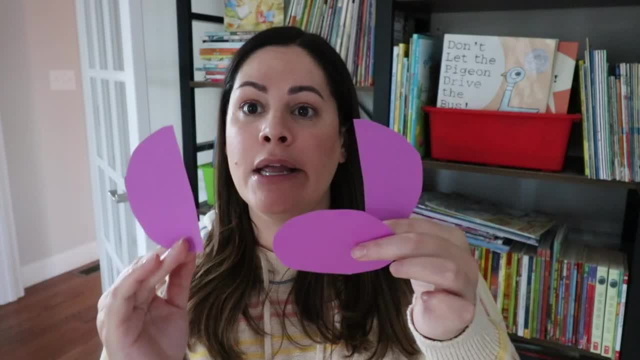 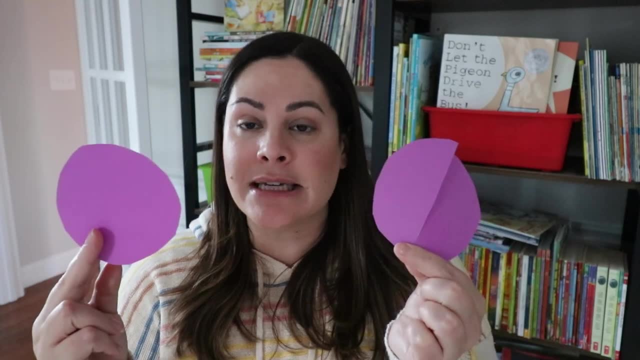 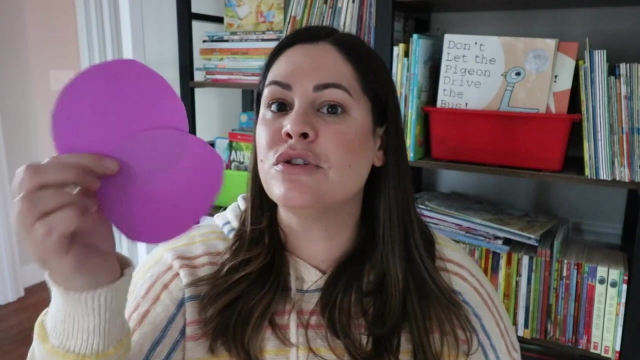 about how to make something. half They talked about what would be equal and what would be not equal, but also they got to do this with their hands. They got to use concrete manipulatives. It wasn't just me talking the whole time. We talked about it, We learned and then we actually did it. So now students should have two. 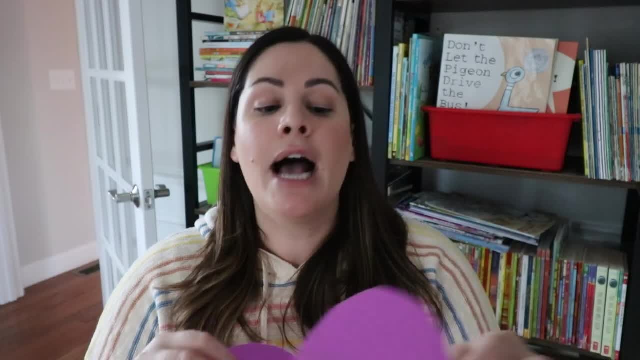 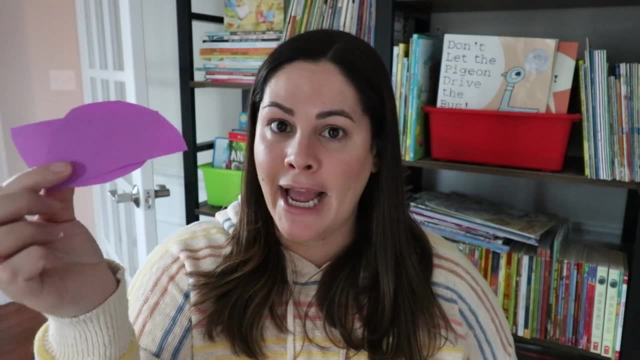 circles and they have their two halves right Their circle that they cut in half. I would have them put this away and use it the next day. On the next day, I'd remind students that we had some circles and we cut one of them in half. I would then ask them to take one of their other. 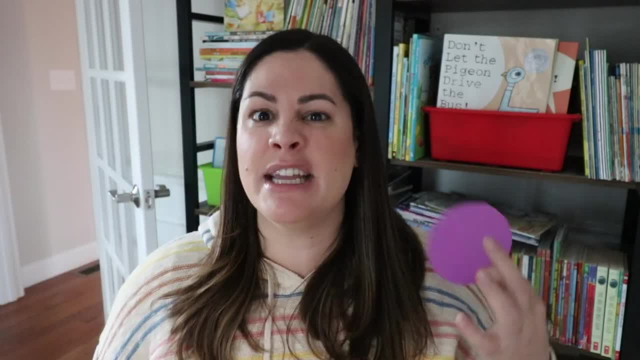 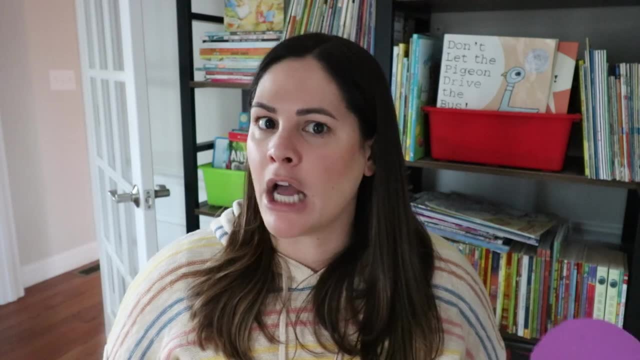 whole circles and I would say, okay, we're going to do the same thing, but today I want to split this circle. I want to partition this circle into four equal parts. How can I do it? Again? same exact process as yesterday, where we are talking it out, We are trying to figure out. 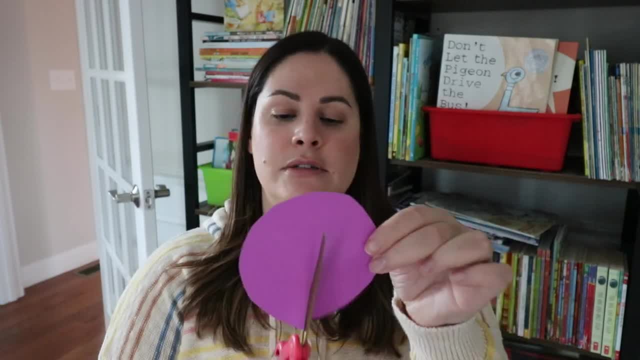 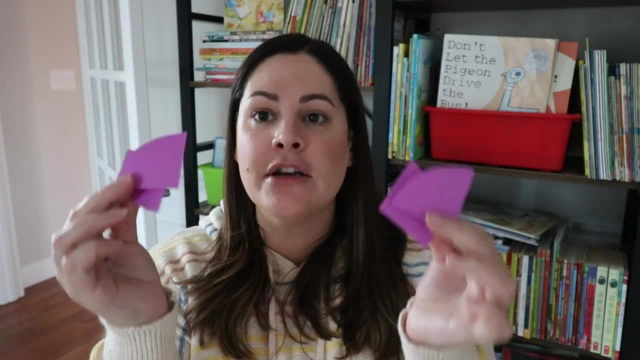 different ways. we can go ahead and cut this into fourths or partition this into fourths, And then, after I do it, my students will do it. So then your students will have four pieces in front of them, And this is when you can also introduce the terms fourths and quarters. We 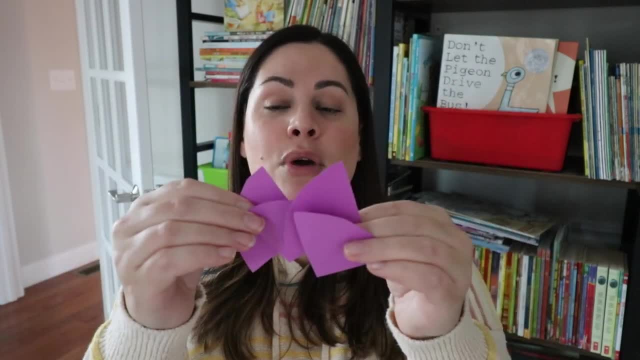 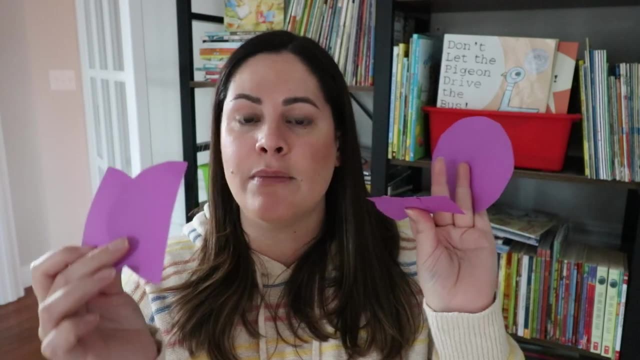 can explain how it's the same thing. It represents a whole being broken up into four equal parts. Now, throughout the days, there is so much more your students can do when they keep these pieces In their little math toolbox. they can talk about the difference between fourths and halves, And 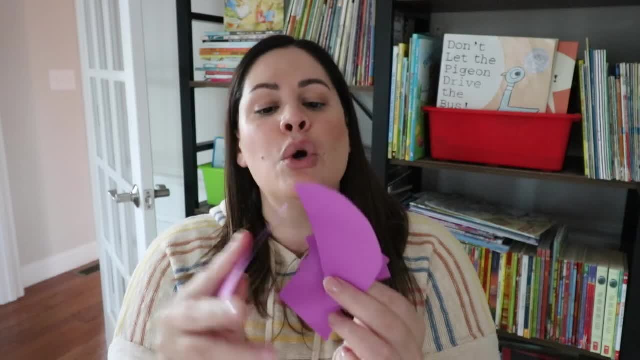 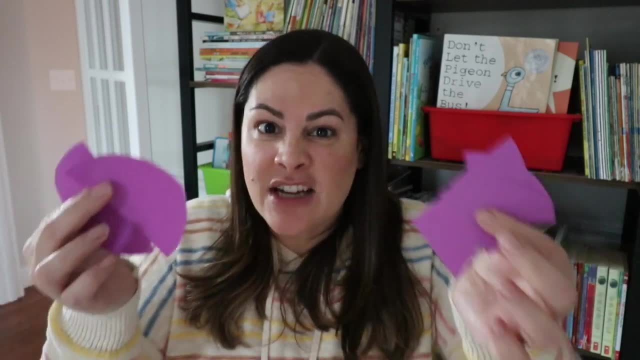 let's pretend they really, really, really wanted a chocolate chip cookie. Would they want one half of a chocolate chip cookie, or would they want one fourth of a chocolate chip cookie? Why, Again, here they're comparing one fourth and one half. but it's not abstract at all, They have it directly. 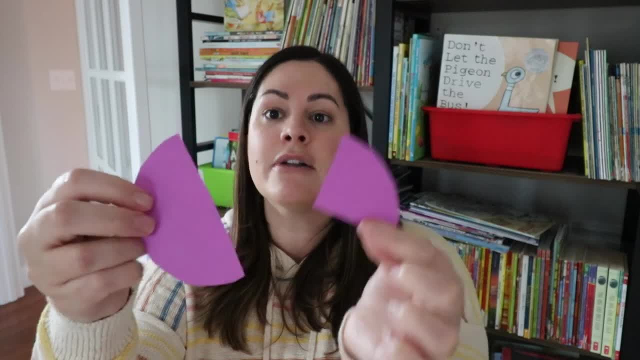 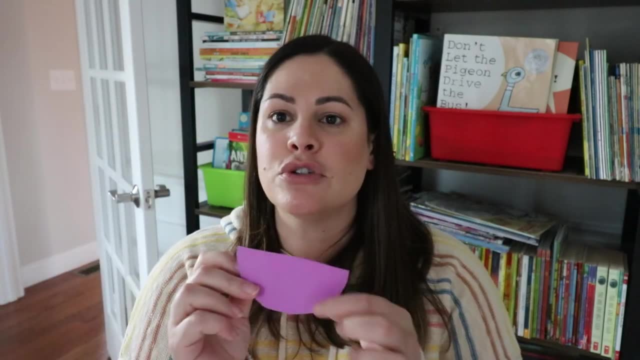 in front of them and they can physically see and compare that this is smaller than this. So if they like chocolate chip cookies, they probably want a half and not a quarter Now to extend this lesson for students to do in small groups or by themselves. 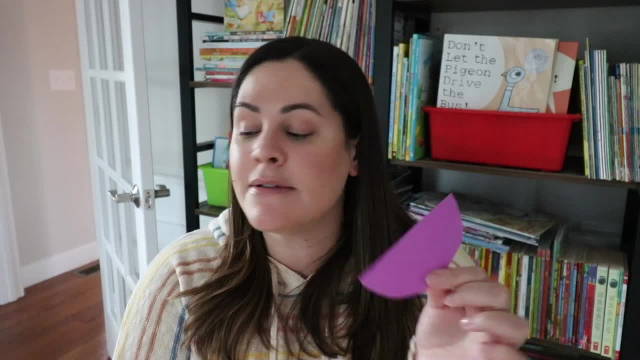 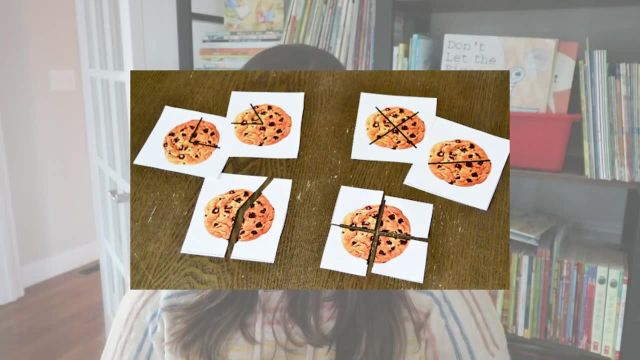 I still like to keep it tactile, have them use manipulatives, And I like to do this with pictures of food. So here's an example of an activity I have called sharing cookies, And students will work with a partner to look at each cookie and decide if the pieces are equal. 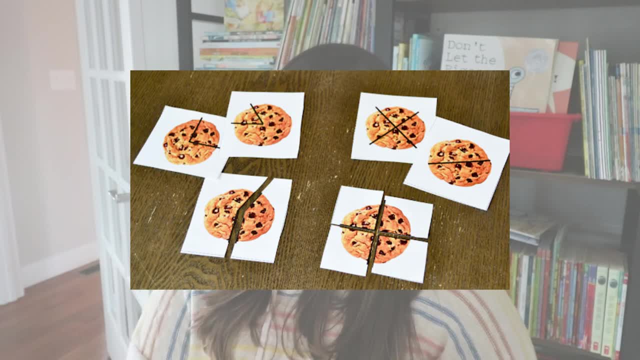 or not. So in this activity all the cookies are divided either into two parts or four parts, But again, they're not always equal. So here students will actually go ahead, take out some scissors. They'll cut that cookie where the line is to determine: is this equal or is it not equal? 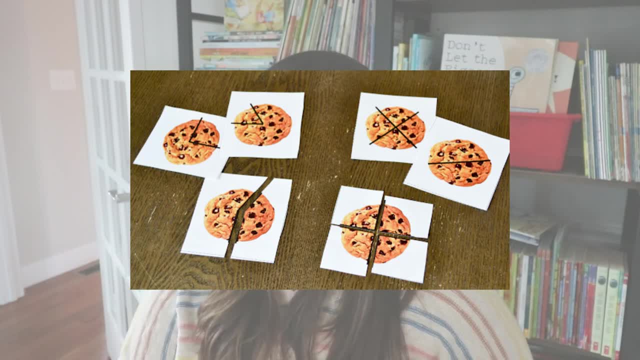 And when they're doing this type of activity I will usually write some sort of sentence on the board that says this cookie is cut into fourths or this cookie is cut into halves, And I challenge students that when they find the ones that are equal, to use one of those. 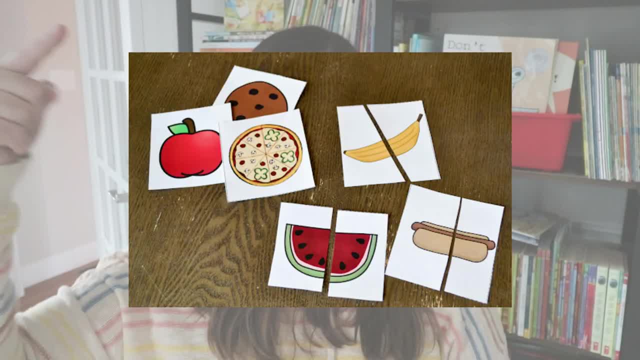 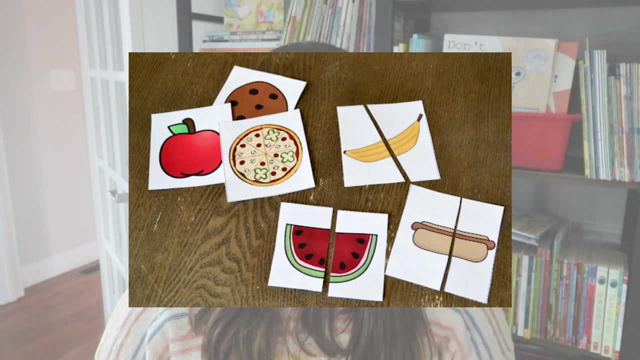 sentences to describe the cookie they just cut. I also have this activity right here called break me off a piece, And this one, instead of just having cookies, has a bunch of different food cards And students are challenged to split that food in half with their partner. So students will work. 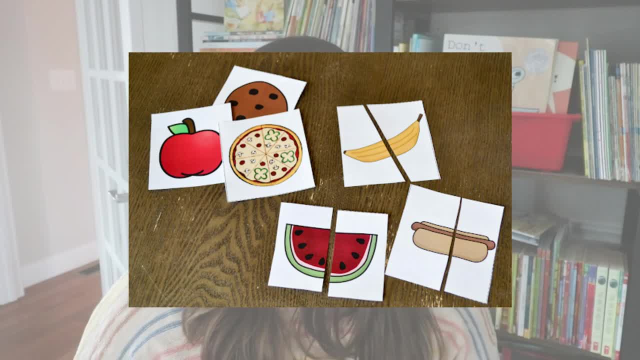 together, kind of like the circle activity we did whole group. but here they'll talk it out: first decide where to go ahead and cut that piece and then decide, okay, did we make it equal or not equal? And what would we change With activity number one? the moral of the story here is to: 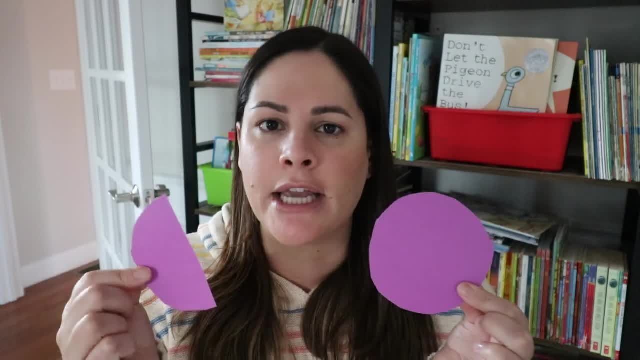 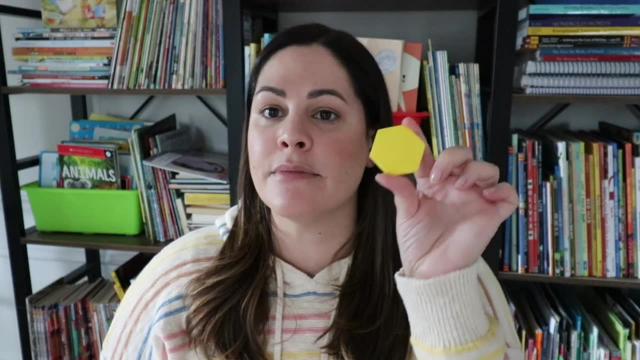 get some scissors, get some shapes and start partitioning. Activity number two is to use pattern blocks to represent fractions. Now, in this activity, students aren't going to be partitioning them themselves, They're not going to cut our pattern blocks, but they are going to. 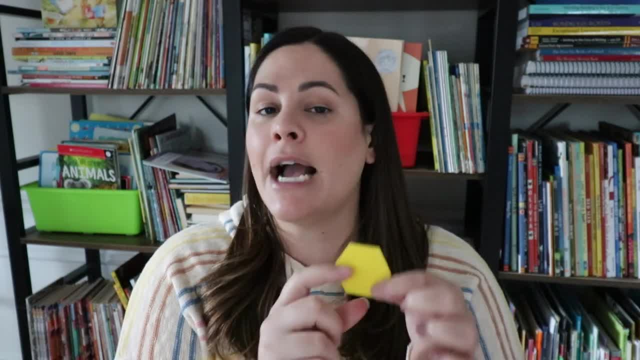 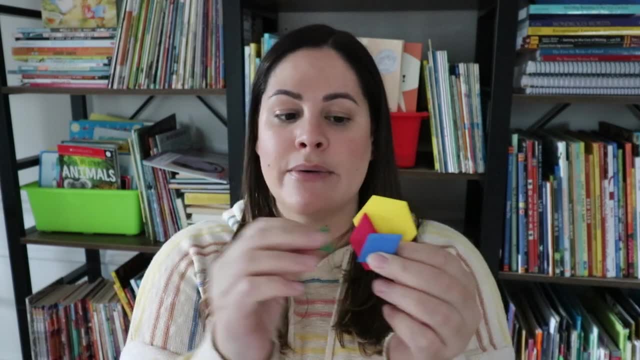 keep it concrete, right? They're going to use manipulatives to actually represent fractions. Now, for this type of teacher guided activity, I would again have the same pattern blocks as my students, So I would let them have a set on their desk and then I would have one under a. 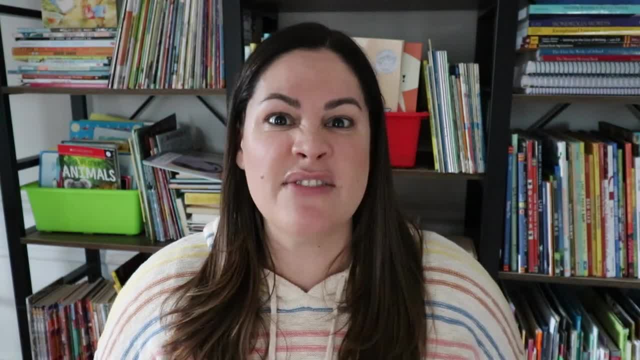 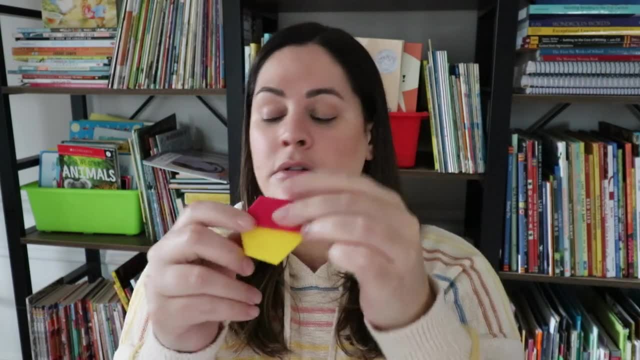 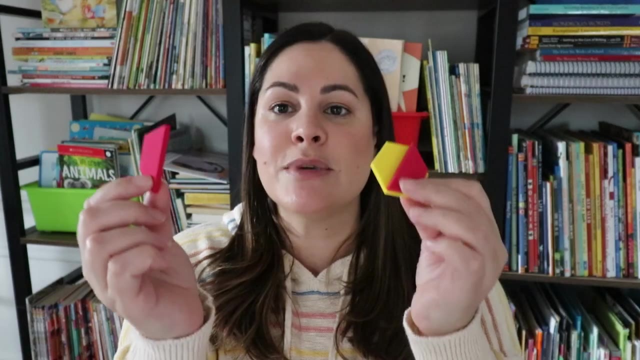 doc, cam or somewhere where all the class can see it, And I would start this activity by simply giving them a question: How many trapezoids fit in a hexagon? And I would want students to figure out that it takes two trapezoids to fill a hexagon. This way, students can actually use the 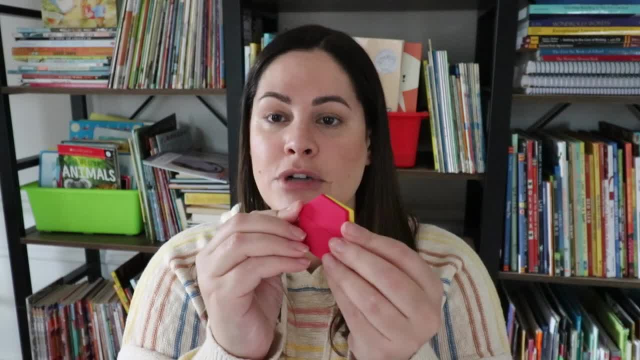 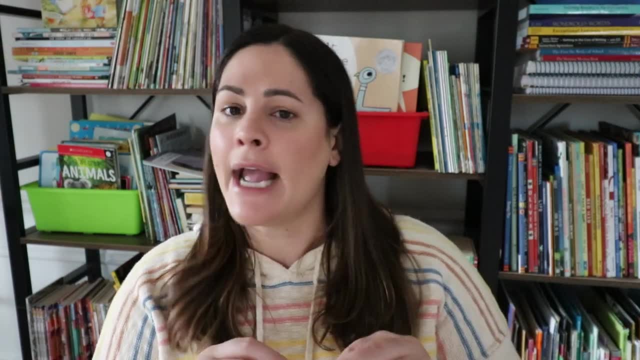 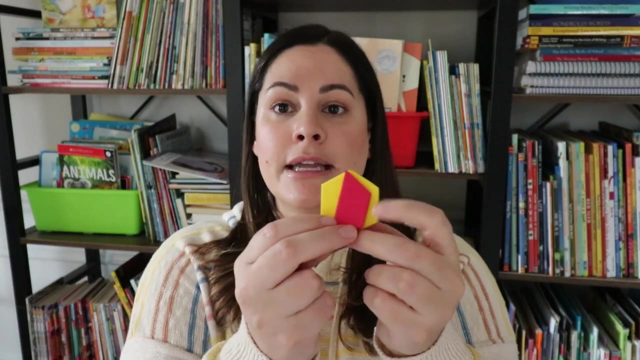 manipulatives, fill it up and see that it does take two trapezoids to make a hexagon, Then I would ask my students to use their knowledge about the word half. So I would say: use the word half to describe how a trapezoid relates to a hexagon, And they might say: one half of a hexagon is a. 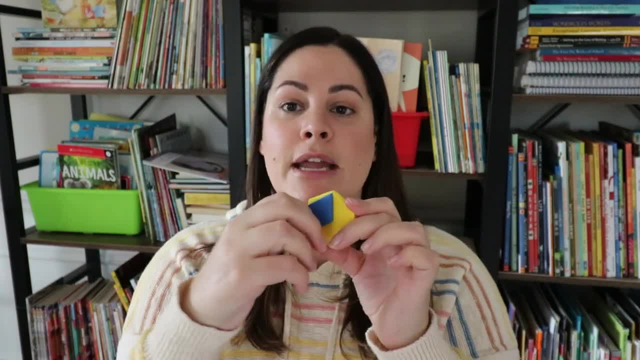 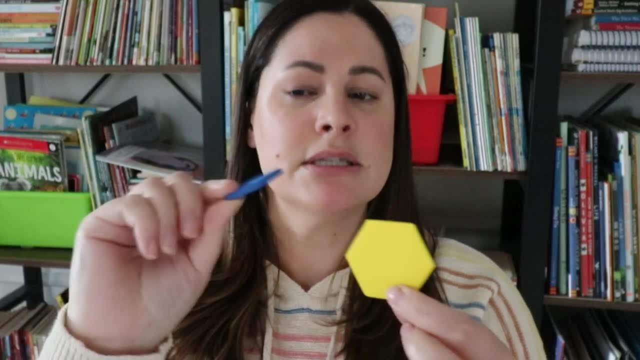 trapezoid. If you're a second grade teacher, you can extend this with a wrong best to talk about thirds, So you can ask your students how many rhombuses. it's rhombuses, right, Not rhombi, definitely rhombuses. How many rhombuses? I think fit in a hexagon. 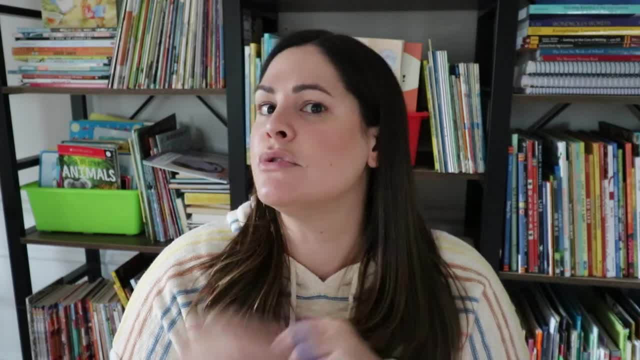 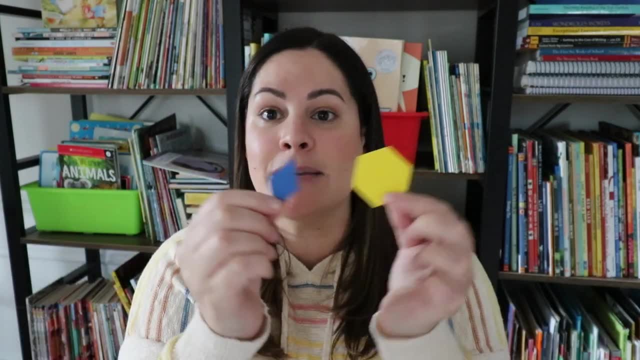 And they will go ahead and see that it's three And then you can say: okay, can you use the word third to describe the relationship between a rhombus and a hexagon? Here we're developing that vocabulary and keeping it concrete. If you're sticking with thirds, we also have triangles. 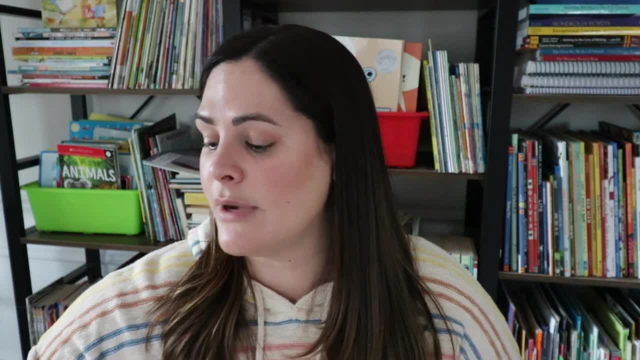 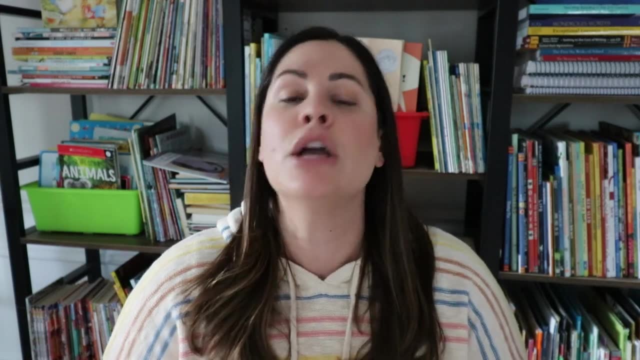 into a trapezoid And then for halves. we also have a rhombus and some triangles. Once you've walked through a few of those with the class, you can have them simply lay out their pattern blocks and then say: show me one half of a hexagon Trapezoid. It might take a little bit. 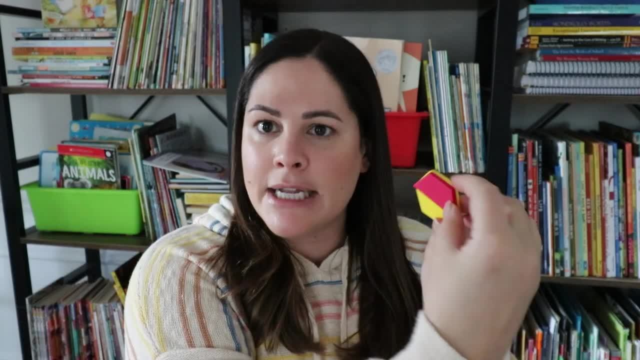 that might not be so quick for some of them. They might need to actually go ahead and manipulate it and see: oh yeah, okay, it was this one, It was this trapezoid. This is one half of a hexagon. 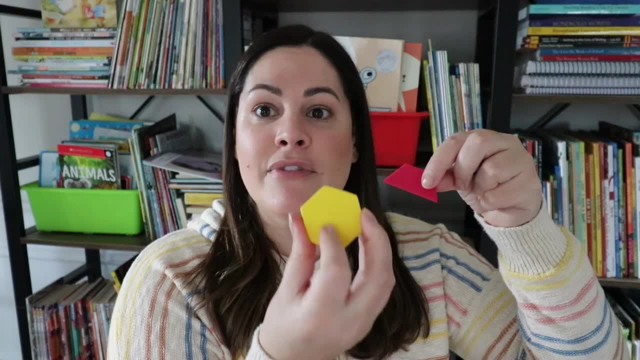 That's great. They are sitting there and they're trying to figure out. they know that half it needs to be broken into two. It needs to cover half. And then they figure out. it's this one. Show me one third of a hexagon. 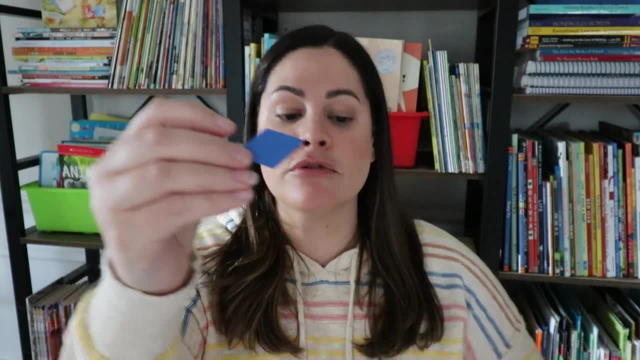 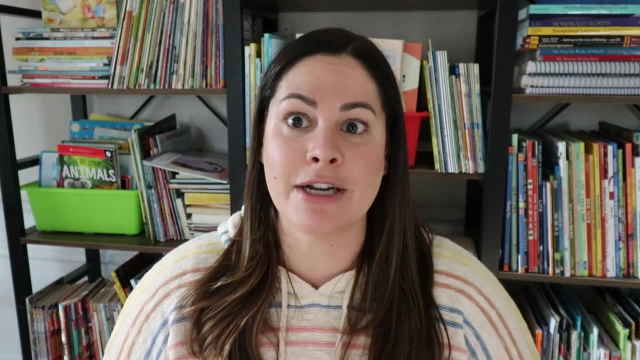 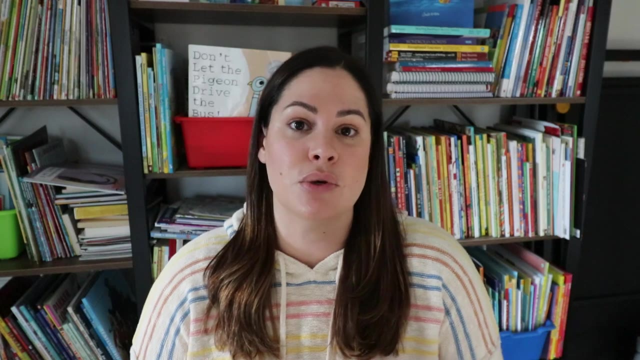 Show me one half of a rhombus. So pattern blocks are a great hands-on way to work on fractions and practice that vocabulary. All right, the first two activities I shared were all about that concrete learning right, And we know how important that is for our students to build those math skills. They 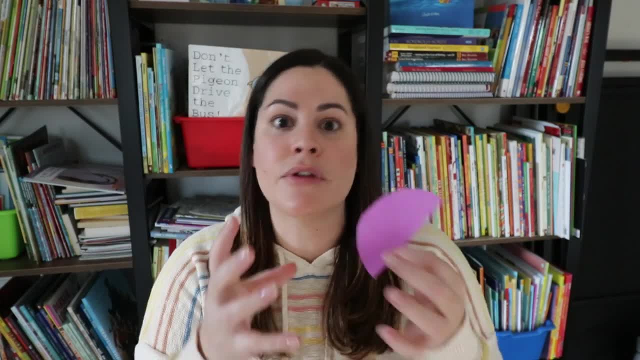 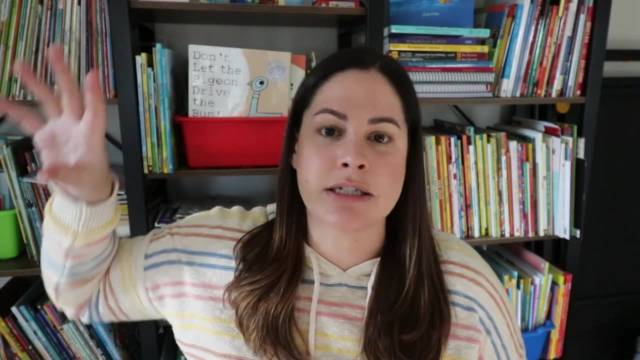 have to be able to understand and show what these math topics actually mean before they can go ahead and represent it And then before they actually understand the abstract. So these are great And I love to have students actually use some scissors- a little fine motor. 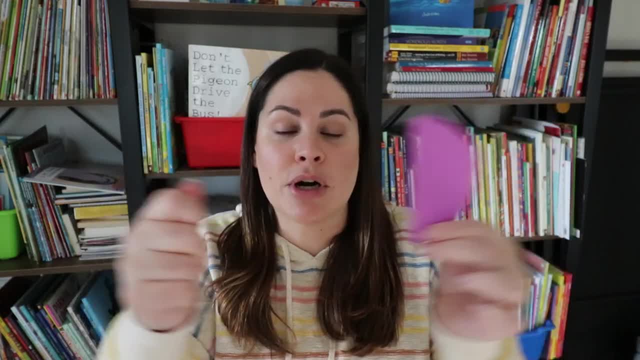 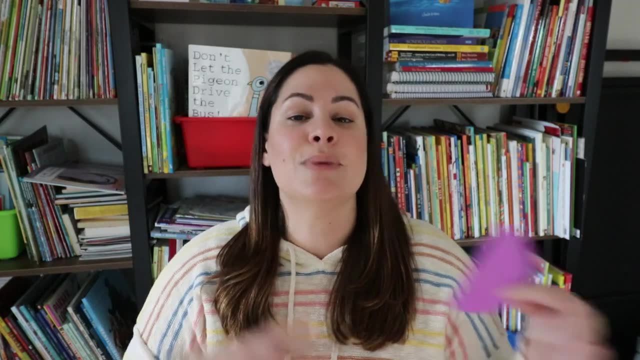 practice, cut something in half and they can actually pull it apart and feel it right. So I also like to have them use Play-Doh. I definitely start with scissors, but then Play-Doh is another way to extend and keep practicing that same type of partitioning. So first we had our 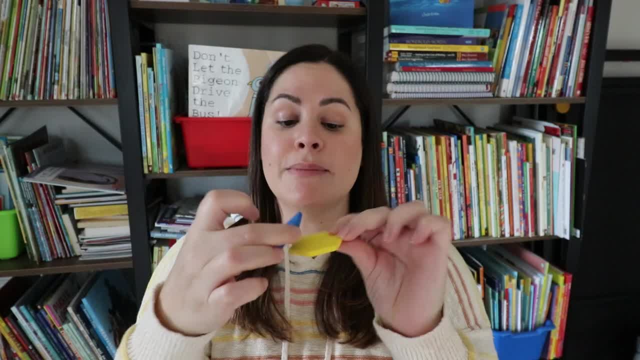 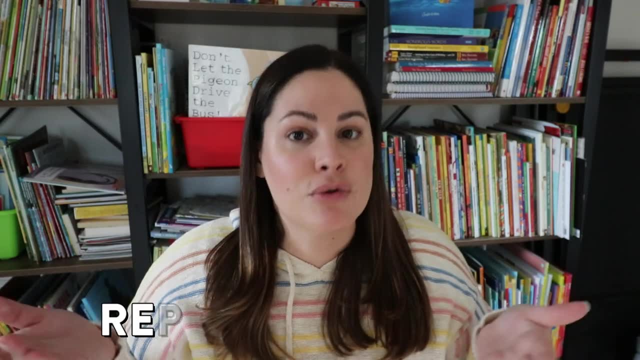 students actually break things apart. Then we also used more concrete manipulatives to show different fractions, while connecting that vocabulary. But now, with activity number three, I want to focus on the representational. When you feel your students have mastered that concrete understanding of? 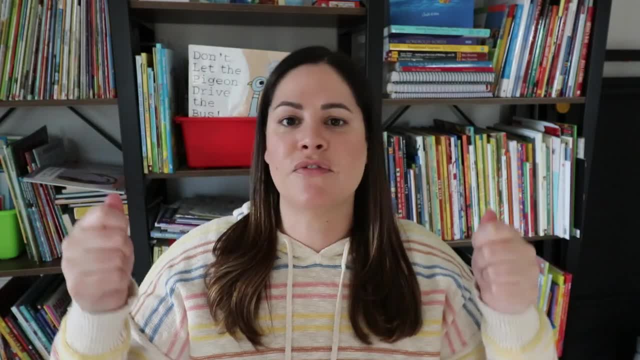 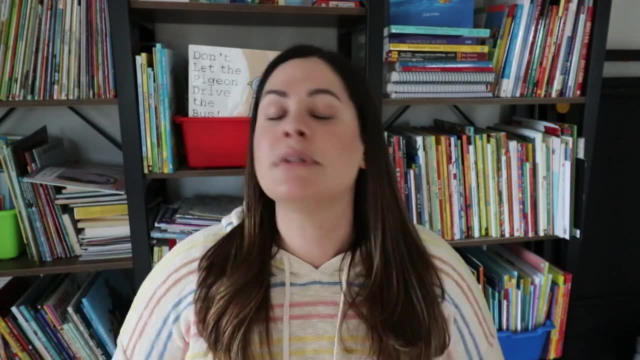 fractions, and they can break something in half, they can break it into fourths, they can show it with manipulatives. let's see if they can identify it in pictures or even create pictures of it. Now there's a few different activities I love for this, The first being a classic math talk. 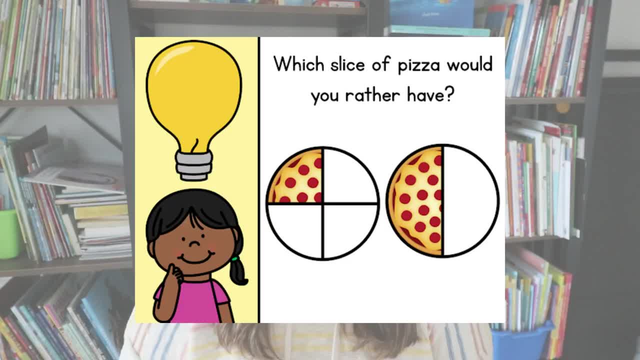 Now here's some examples from my geometry math talks that I actually just came out with. I have an entire bundle filled with tons of different math talks for kindergarten first and second. these are the geometry ones. So here we have pictorial representations of fractions. 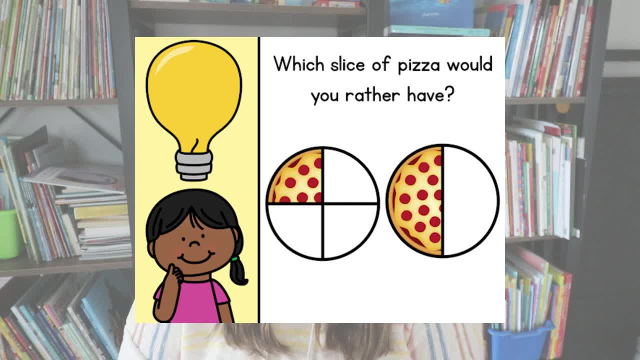 So here's an example of two slices of pizza and I would ask: which slice of pizza would you want and why, right They have to explain. So here they have to recognize that, okay, this slice over here, this pizza is broken into fourths and this pizza over here is broken in half. 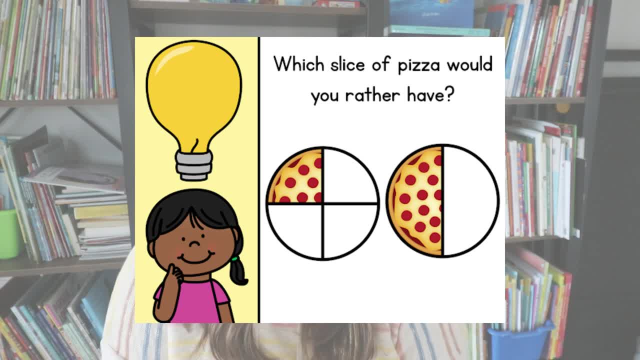 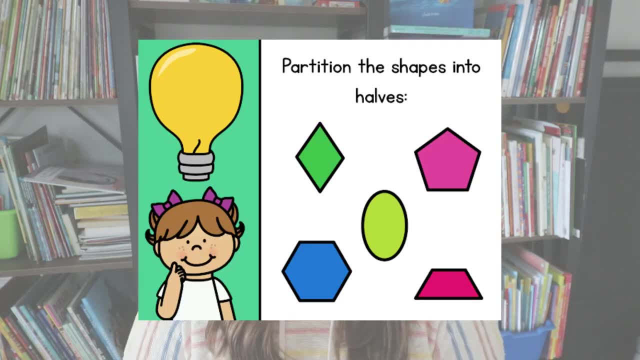 so which slice do I want? If I'm feeling really hungry, maybe I want the half. If I'm not as hungry, maybe I want the fourth. They have to explain it using what they know about these fractions. Another example of a math talk I would use with my: 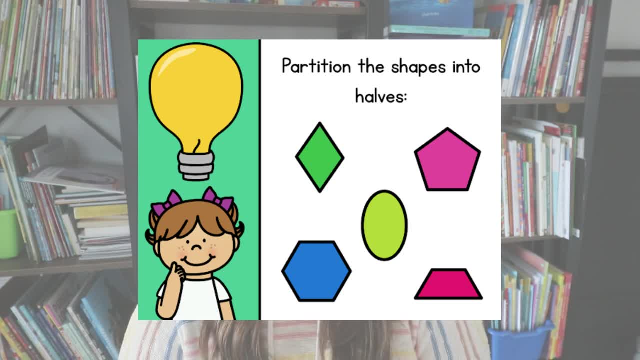 students would be this right here: Partition the shapes into halves. I always display these on the smart board, so students would come up with their marker and they would draw a line to break these shapes in half. And, as you can hopefully see, with most of these there's going to be a few different. 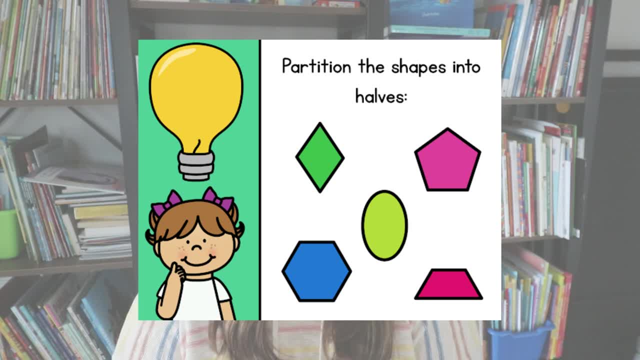 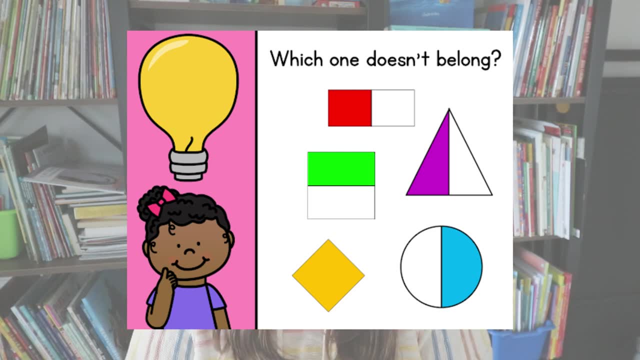 ways they could do that, and that's what we will talk about during this math talk. Lastly, here's another quick example, which one doesn't belong Here. we have four images that all represent one half of a shape, And then we have two shapes that represent one half of a shape, And then we have 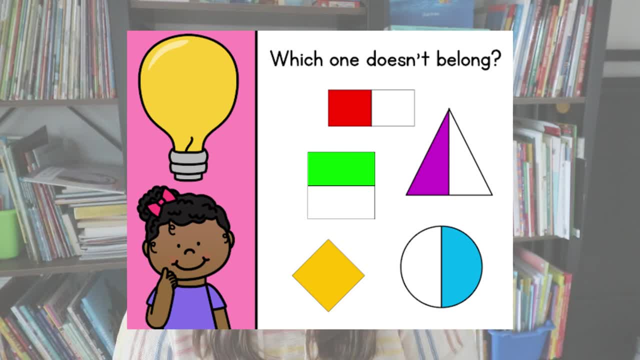 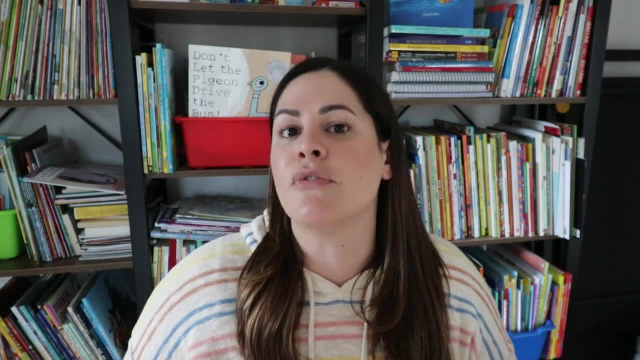 this other one down below that's fully shaded in representing a whole. So students have to explain which one doesn't belong and why. Through those math talks students are deepening their understanding of fractions and what we've already learned. In some of them they're actually coming. 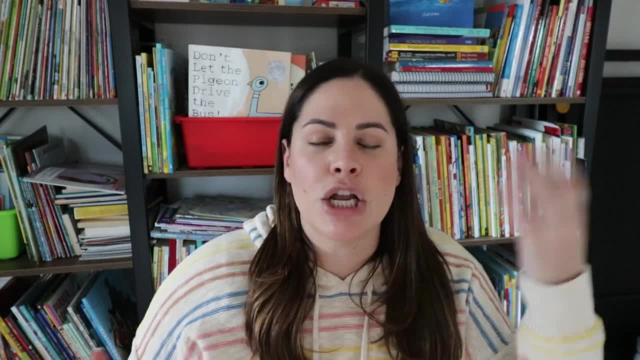 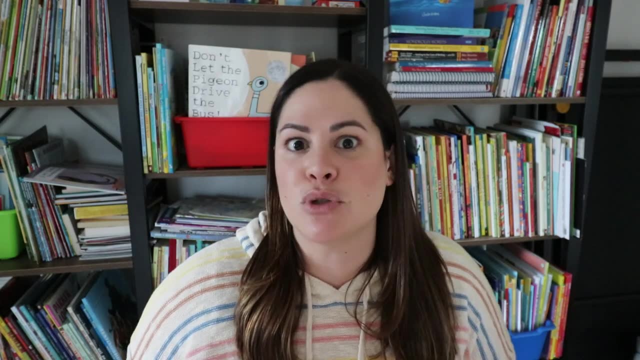 up in partitioning shapes, In other ones they're comparing, you know a fourth and a half, or they're recognizing what's different about these fractions. So it's a great way to really deepen their conceptual knowledge. Another easy activity to help with the representational aspect of fractions: 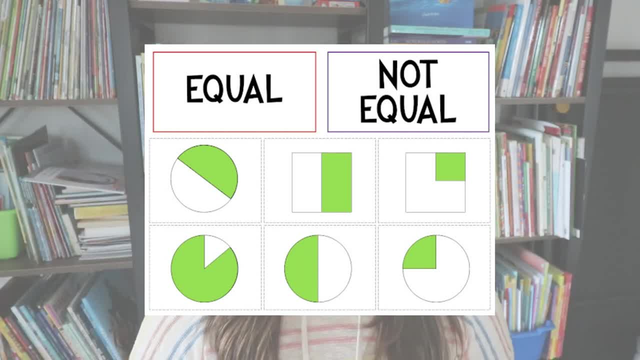 are to do some sorts Here. we have a simple equal versus non-equal sort, where students will have to look at the shapes and how they are broken apart and determine are these pieces equal or are they not equal, and sort them. I always start with a sort like that, one where students will work either 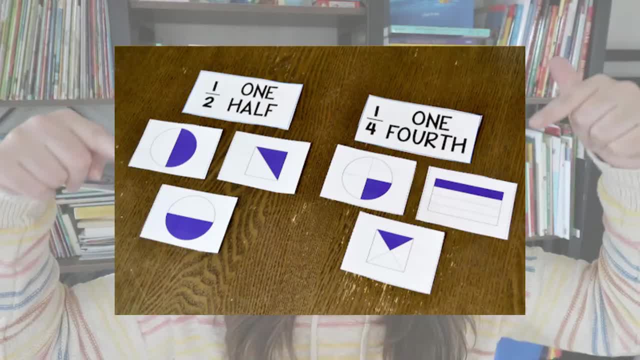 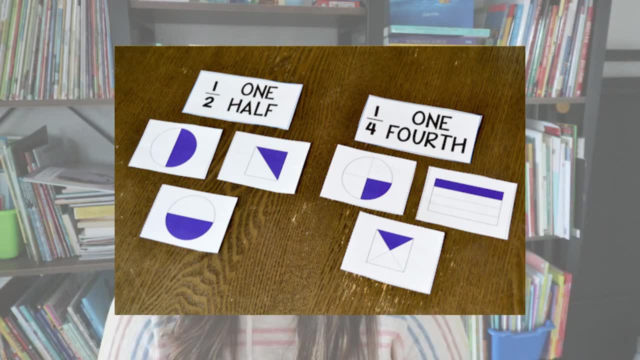 with a partner or independently to do that. And then we move on to this one right here where students have to decide: does this represent one half or one fourth? Now, it's important to note that here in the headers you do see that abstract, uh, version of a fraction. right, We have one two. 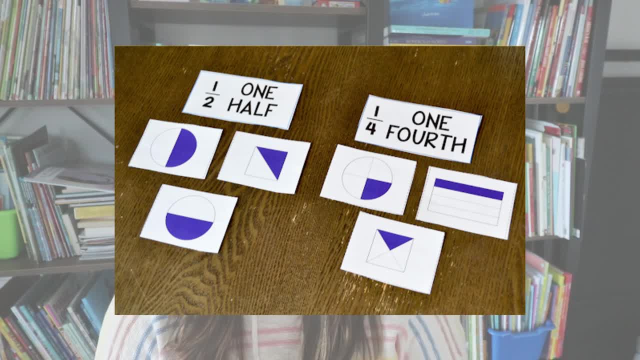 one over two and one over four, to show one half and one fourth. By this point, if students are working independently, I don't see much harm in showing them and exposing them to this abstract part, As long as I know that students don't have to master that and I don't introduce it too early. 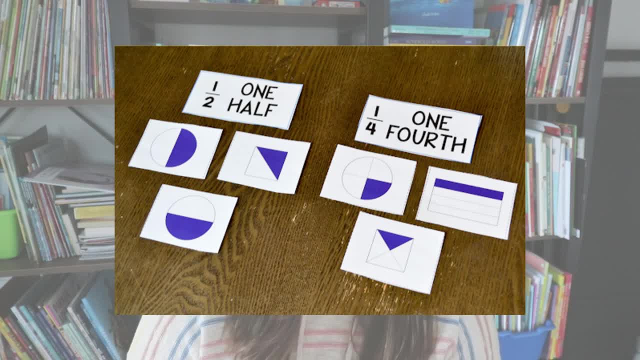 there's really no harm in allowing them to see what one half looks like, when they are also comparing it to pictures of things that are broken in half And the same with one fourth. So here, students will simply flip a card, They will look at the fraction and determine. 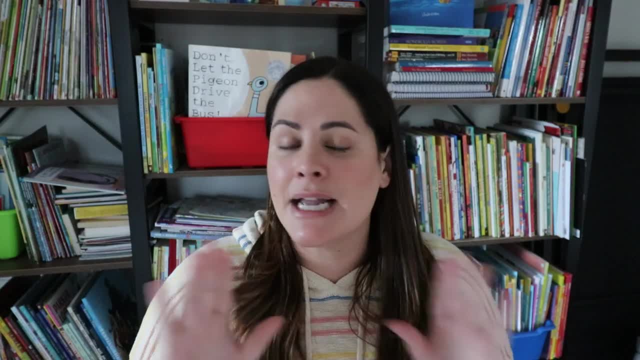 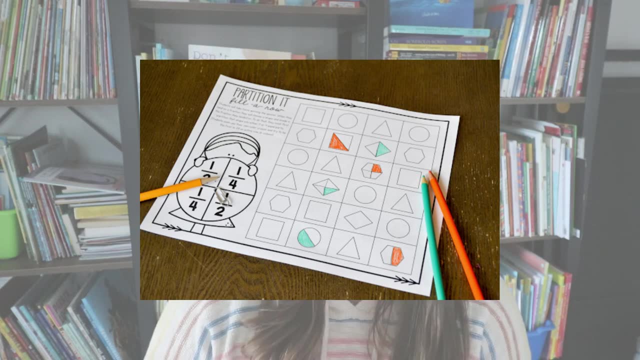 is this showing one half or one fourth, and sort it. Lastly, I always love some print and play partner games, so I have some spinner games that students can play as well. This one is called partition it, and students will spin the spinner down on the left hand side and then they will. 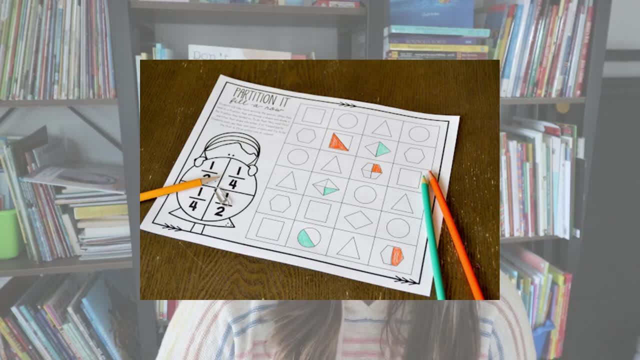 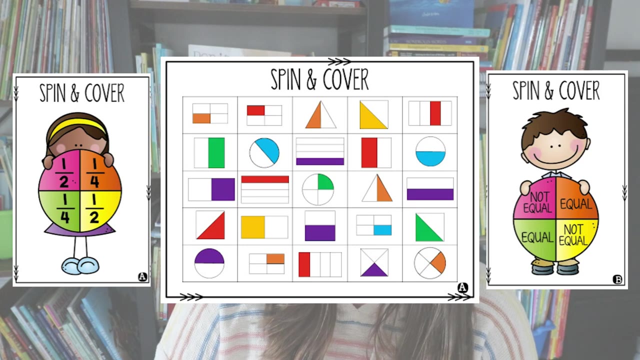 find a shape to either partition in half or partition into fourths. They can choose the shape, but here they are practicing not only recognizing the difference between one half and one fourth, but again partitioning it themselves. So they have to draw the line and shade in that fraction. I also have this spin and cover game where students will again review. 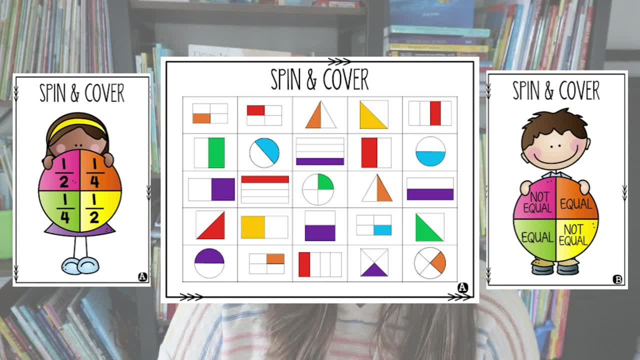 equal and non-equal parts, as well as the fractions one half and one fourth. and here they will, instead of actually partitioning it themselves, they will go ahead and just identify it. So they will spin on the left and cover up something in the grid that matches All of those sorts and the spinning. 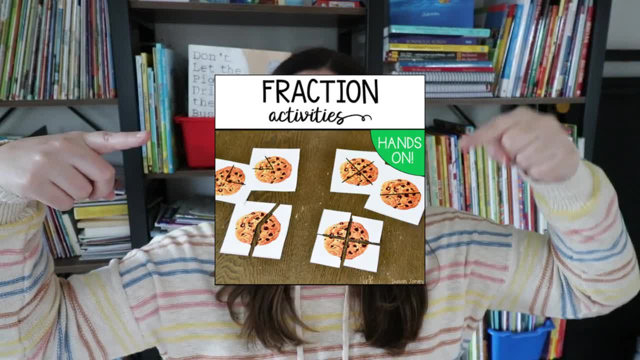 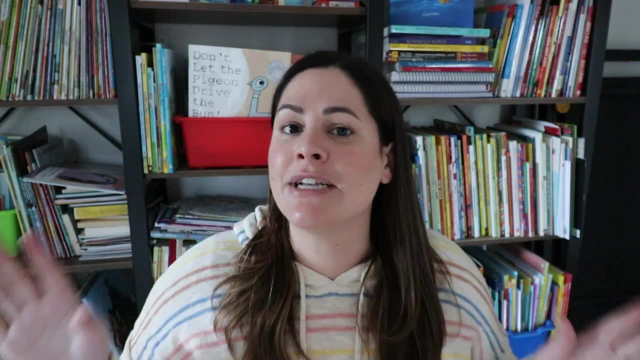 games are actually included in my hands-on fractions unit. that looks like this over on TPT. I will link that down in the description along with my number, talks and anything else I mentioned in this video. But just to recap one last time: you want to focus on concrete and 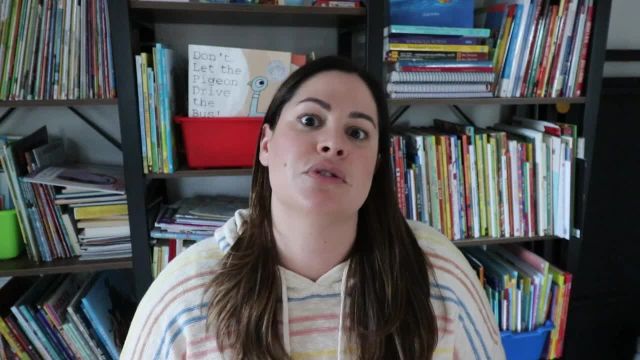 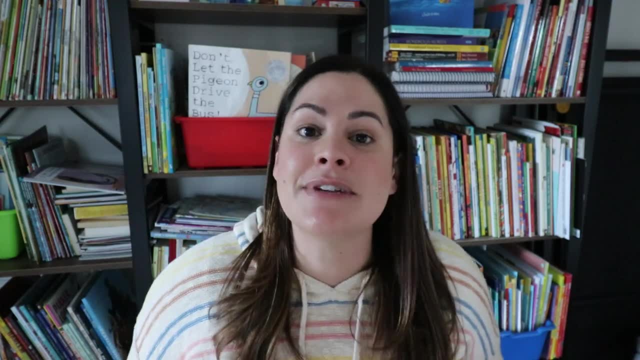 representational activities that will really help your students build those foundational skills so they understand what fractions really mean. I hope if you are teaching fractions soon, you can take some of these ideas and activities to use with your own students right away, As always, if you. 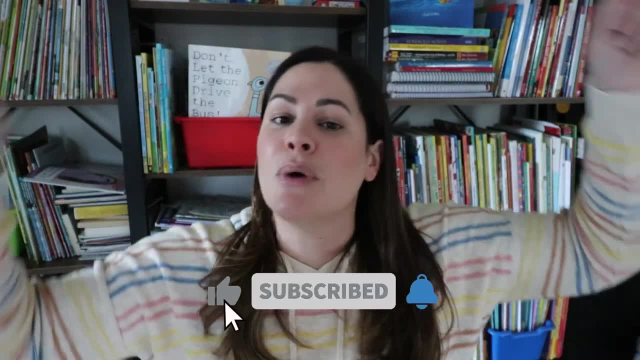 did enjoy this video. please give it a thumbs up, so I know. Make sure you are subscribed to my channel and click that bell. that way you're notified of every new video. See you in the next one. Bye. 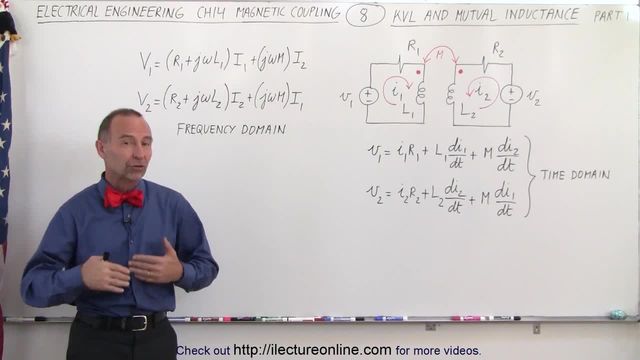 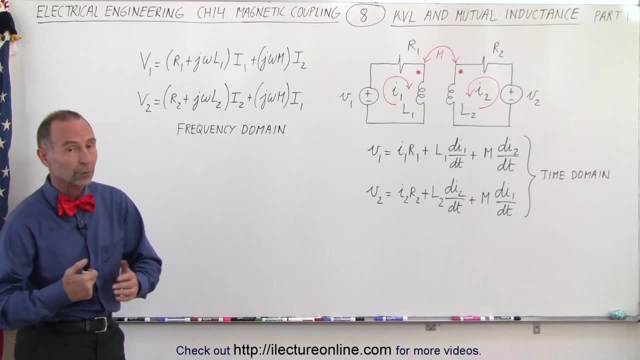 Welcome to our lecture online. If we're now going to take a look at circuits using the Kirchhoff voltage laws, how do we deal with mutual inductance? Well, we do it as follows. Let's say we have two circuits that are coupled together through mutual inductance. Notice that. 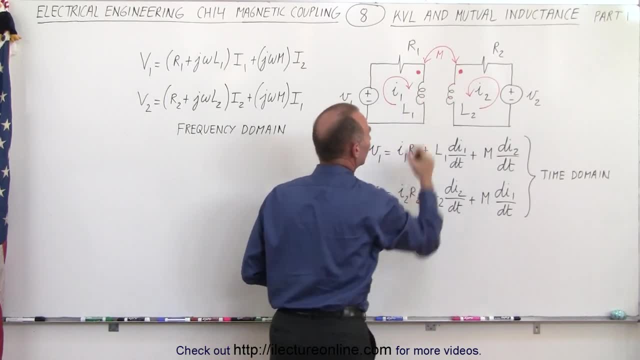 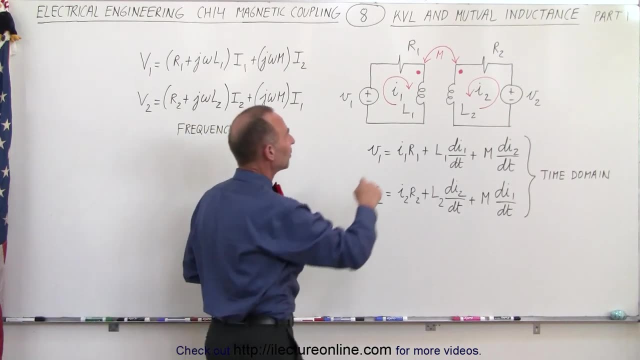 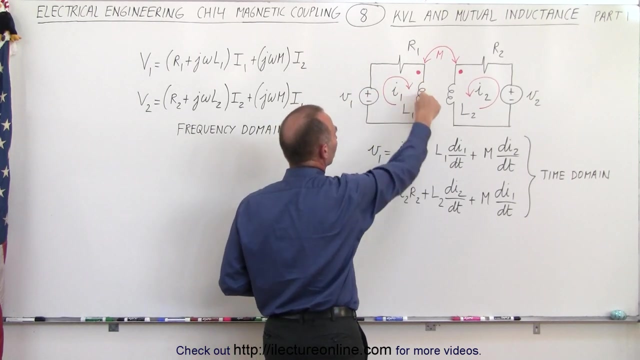 they have the same what we call coupling on the same side of the inductor so that there is a mutual aid in the coupling. And then we can see that if we go around the circuit and we add all the voltages, that the voltage across the voltage source must be equal to all the voltage drops. 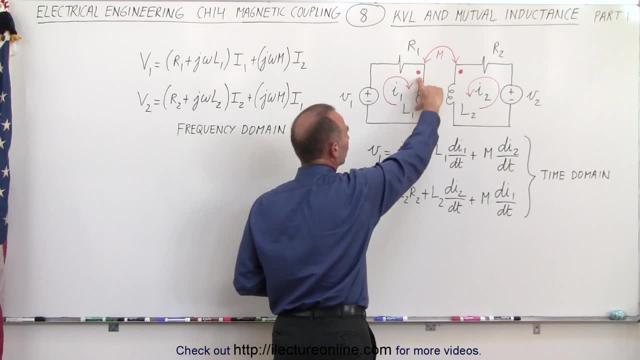 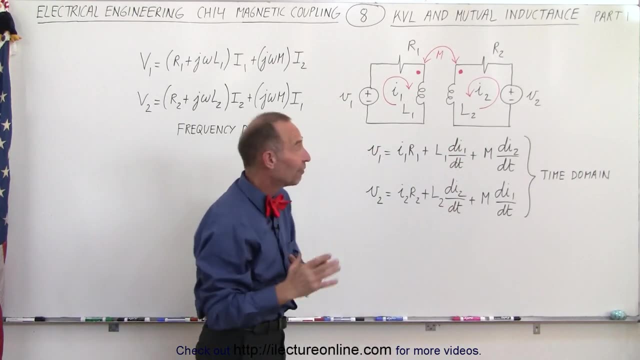 Notice: we have a voltage drop across the resistor, we have a voltage drop across the inductor, so it'll be I times R plus the self-inductance times di dt. But we also have a voltage drop due to the mutual inductance between the two inductors, so we add an additional term. 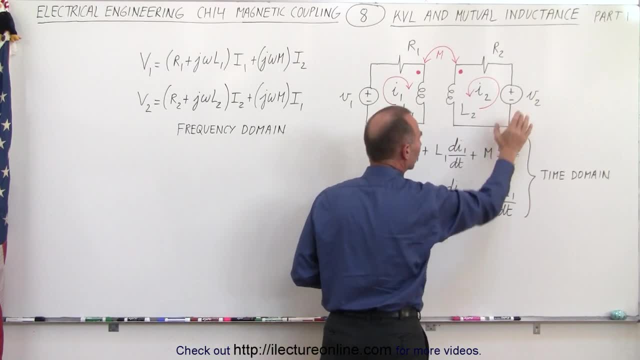 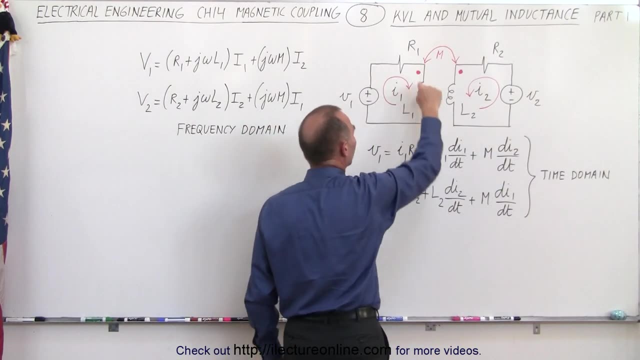 the mutual inductance Times, the rate of change of the current in the other circuit with respect to time. So you can see that there's one additional term that we need to add to the total voltage as we go around the loop. Same when we go around the second circuit. Notice that's going to be the sum of the voltage. 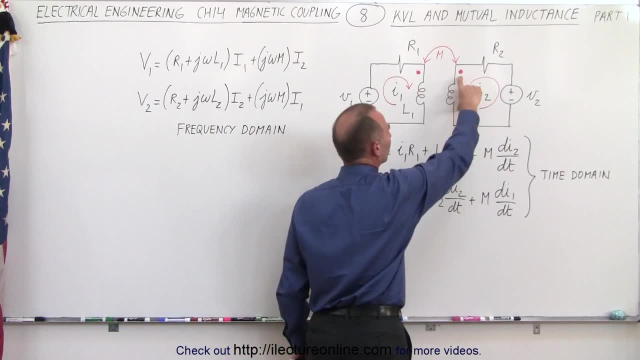 drop across the resistor. the voltage drop across the inductor due to the self-inductance plus the voltage drop across the inductor due to the mutual inductance. And that of course, since the coupling here is the same on the same side of the circuit.